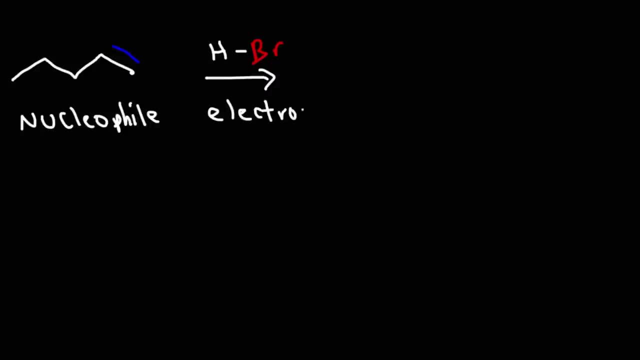 HBr is going to be the electrophile in this reaction. It's going to accept a pair of electrons. The nucleophile is like the Lewis Base. The electrophile is basically the Lewis acid. Now, to show the mechanism, the arrow is always going to start from the nucleophile and it's going to go to the electrophile. 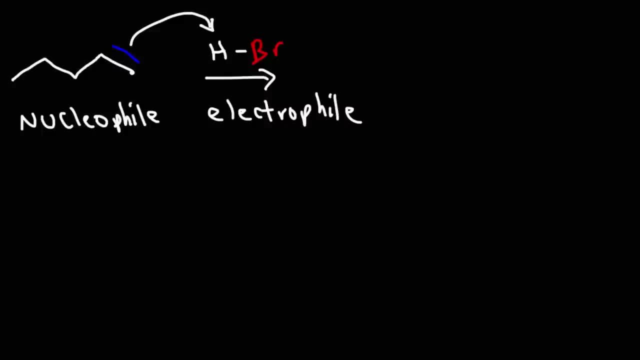 Now the reason why the nucleophile, in this case the alkene, is going to react with the hydrogen in HBr is because hydrogen is partially positive. bromine is partially negative. Bromine is more electronegative than hydrogen. As a result, you have unequal sharing of electrons. 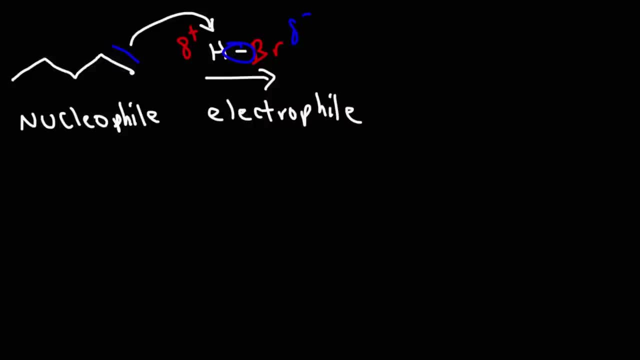 in this bond. Because bromine is more electronegative, it's going to pull those electrons in that covalent bond closer to itself, And so bromine is going to acquire a partial negative charge. hydrogen is going to be partially positive, So it's going to be deficient in. 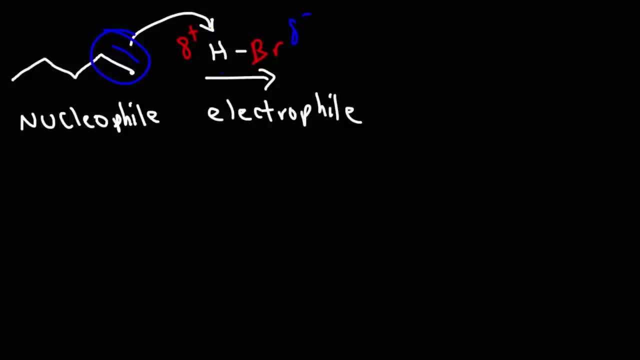 electrons. The nucleophile, being electron rich, is attracted to this partially positive hydrogen atom, And so it's going to react with the hydrogen part in HBr. Now the arrow represents the flow of two electrons. What's going to happen here is the pi bond is going to break, And those electrons 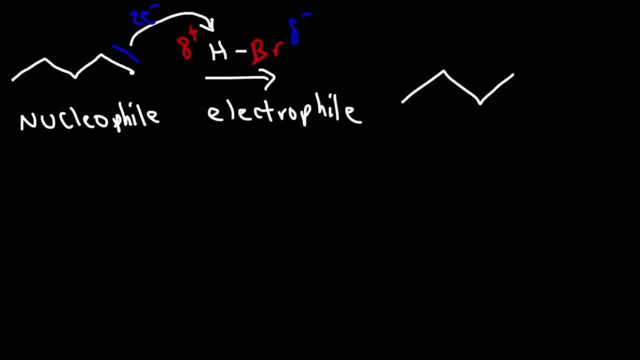 will be used to form a hydrogen bond, And so hydrogen is going to react with the hydrogen bond to form a new bond between the primary carbon and the hydrogen. Now here's a question for you: Why does the hydrogen go on the primary carbon and not? 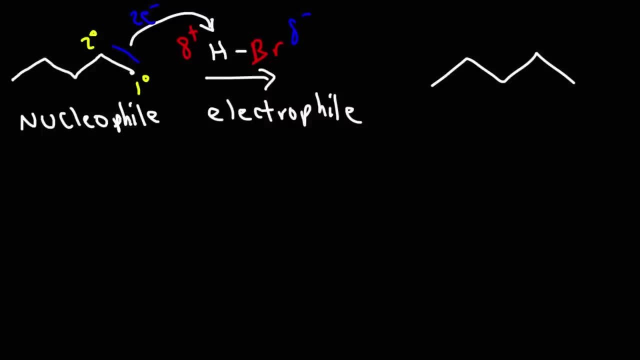 the secondary carbon. Why should we put the hydrogen on the primary carbon? If we put the hydrogen on the primary carbon, we're going to get a secondary carbocation. If we were to place the hydrogen on the secondary carbon, we're going to get a primary carbocation. 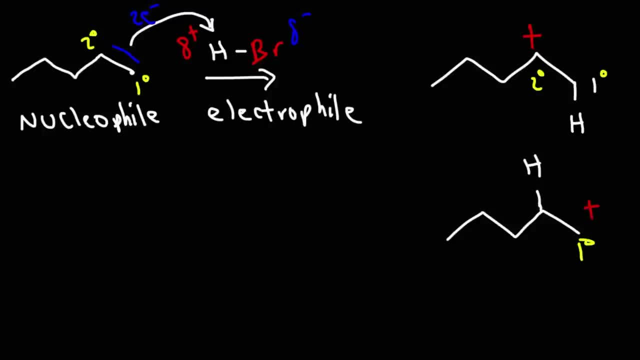 Now, the reason why this doesn't happen is because primary carbocations are less stable than secondary carbvatines, So you need to know that Tertiary carbocations are more stable than secondary carbisaes, which are more stable. So it's important to know two things about. this. The first is that the higher the level of carbon in an anyway ignition, the higher the losses of the OHlagenin on a carbo stay come from the other side—that the more stable than primary carbocations. So the reason why the hydrogen goes on the less. 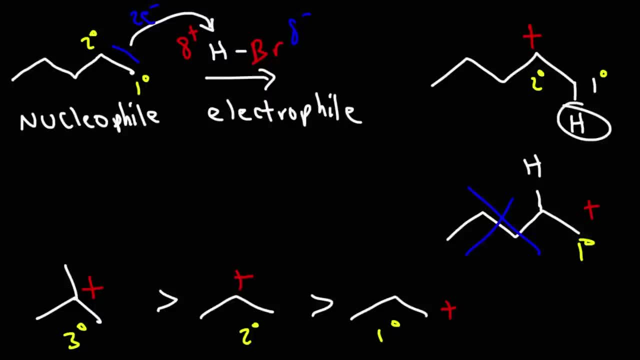 substituted carbon is because it forms a more stable carbocation intermediate. Now let's go back to the reaction. So after this pi bond breaks, those electrons are used to form the bond between carbon and hydrogen. And in order to form a bond between carbon and hydrogen, this bond must break as well. Now, because bromine 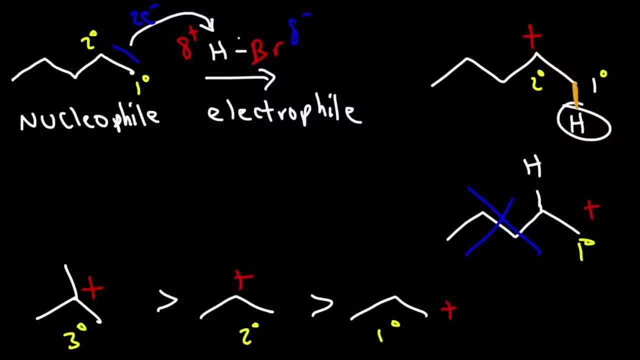 is more electronegative than hydrogen. when this bond breaks, the electrons are going to go towards the bromine atom. Initially, before that happens, bromine has three lone pairs. Now it's going to have four. So here we have our secondary carbocation intermediate with our newly 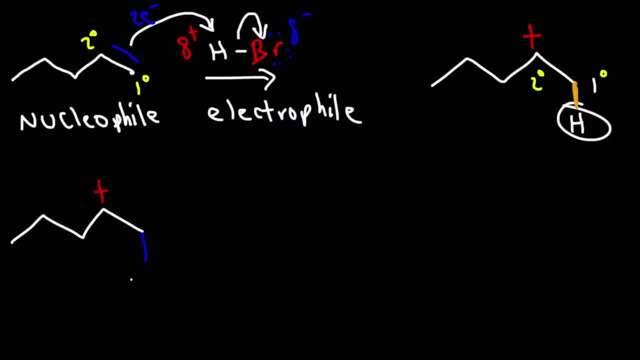 formed CH bond And now we have the bromide ion in a solution next to the carbocation. Now the bromide ion has a negative charge and we know opposites attract. So it's going to be attracted to that positive charge, charged carbocation. So to show the mechanism, we're going to draw the arrow from the nucleophile. 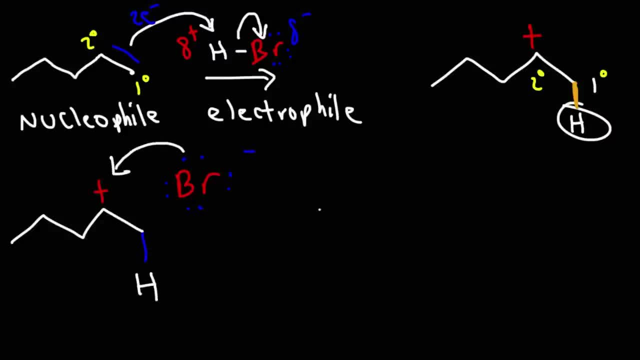 to the electrophile from negative to positive. So bromine is going to use a lone pair or two electrons to form a sigma bond between the secondary carbon and itself, And so this is how we're going to get the final product. By the way, every single bond contains a sigma bond. 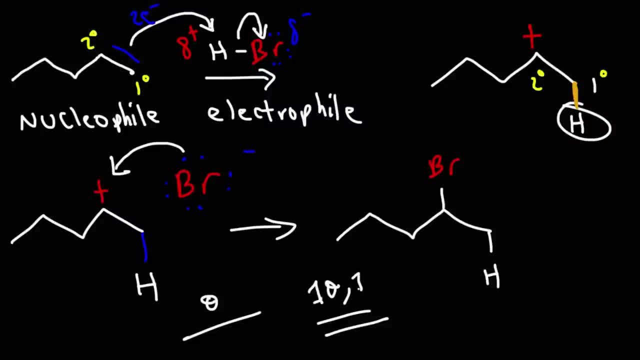 A double bond has one sigma bond and one pi bond. A triple bond has one sigma bond, two pi bonds. Sigma bonds are stronger than pi bonds. It's easier to break a pi bond, but it's harder to break a sigma bond, So alkenes are therefore quite reactive. 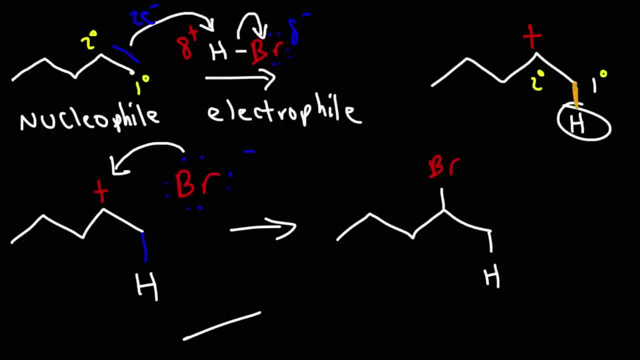 because they carry a pi bond which is relatively easy to break. Now let's go back to this part. The bromide ion can attack the carbocation in two different ways: From the front, or it can attack from the back. Because it can approach the carbocation in both ways, we can get a mixture. 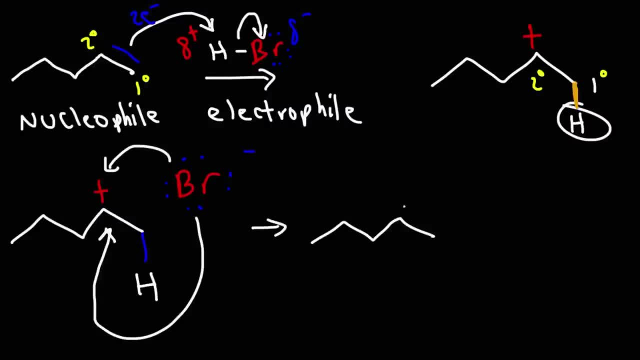 of products. So we can get both the R and the S isomers in this reaction. So this reaction is regioselective Because the bromine atom will selectively be added to the secondary carbon and not the primary carbon. So we have a regioselective reaction. 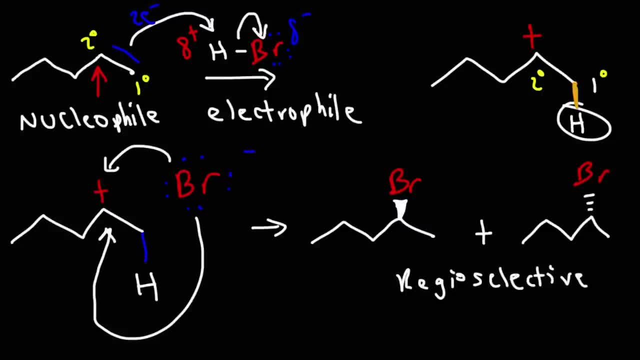 Now, this reaction is not stereoselective. There's no stereospecificity in this reaction because we get a mixture of stereoisomers. We don't get one stereoisomer over the other, we get both. So it's not stereoselective. 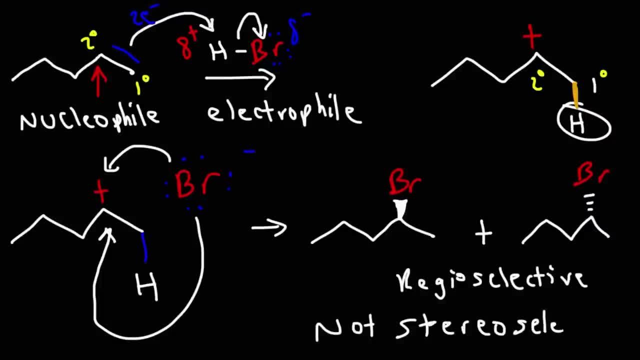 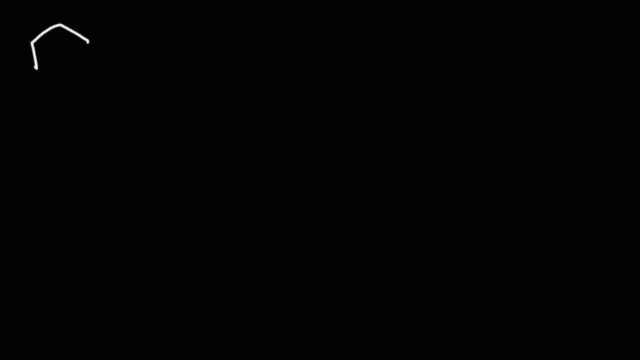 But it is regioselective. Now let's work on some practice problems. Go ahead and predict the major product for each of the following reactions in this example. Feel free to pause the video and work on these examples. Just start with the involution of the firstiders on your unit. 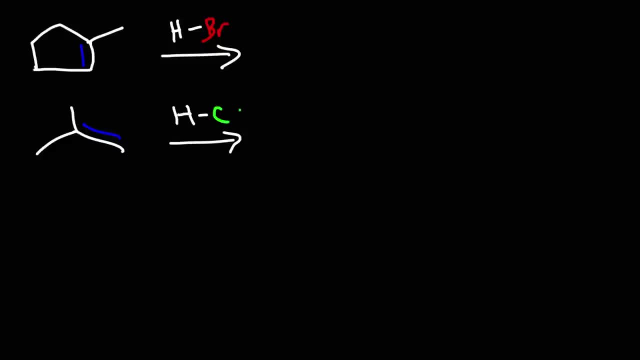 And maybe then go on to the next one. Just imagine that the 활동 of the butexyl airplanes at this moment, Just look at what is happening. So what will be the major product? for the first example, Compared with a bromine atom, where is it going to go? 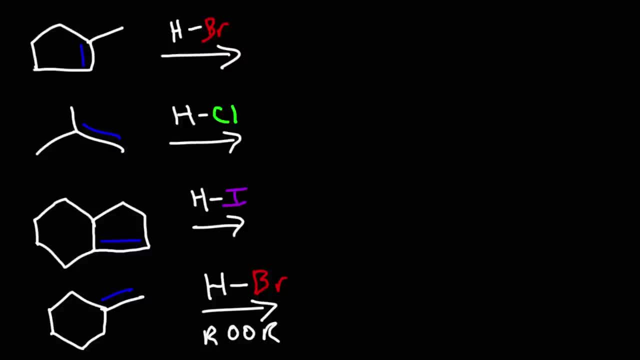 Whenever you mix HBr with an alkene, the bromine atom is going to go on a more substituted carbon atom. So this carbon is secondary because it's attached to two other carbon atoms, and this one is tertiary because it's attached to three other carbon atoms. 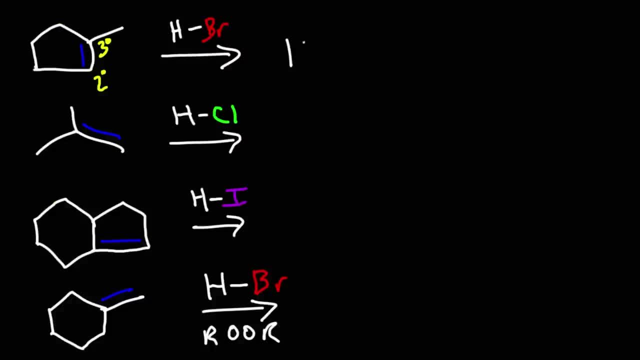 The double bond is going to turn into a single bond because this is an electrophilic addition reaction. The hydrogen is going to go on a secondary carbon, The bromine is going to go on a tertiary carbon. This reaction is regioselective. 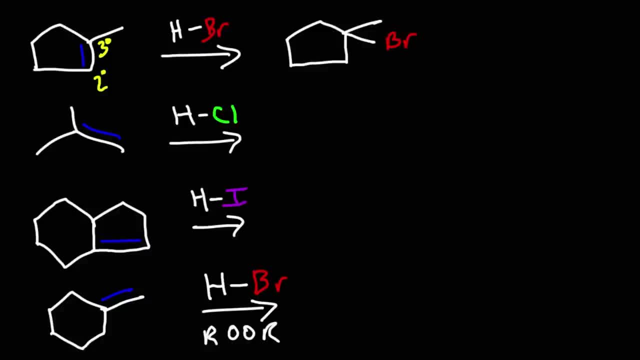 It proceeds away from our carbonyl carbon addition. For the next one, the same is true with HCl. The chlorine is going to go on a more substituted carbon atom. This carbon is primary, It's attached to one carbon, and this carbon on the other part of the double bond is tertiary. 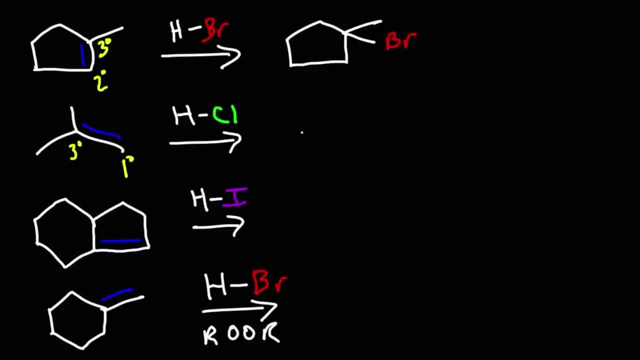 It's attached to three other carbon atoms. Okay, So we're going to break the double bond and put the chlorine atom on the tertiary carbon. There's no need to show the hydrogen in this example. You can just leave your answer like this. 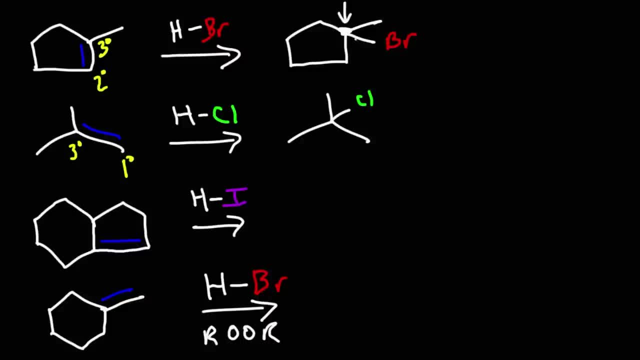 Now, this carbon atom here is not chiral because this side is equivalent to that side. For this carbon atom it's not chiral either because we have three identical methyl groups. So we don't need to show tertiary. We're going to show stereochemistry for the products of the first two examples. 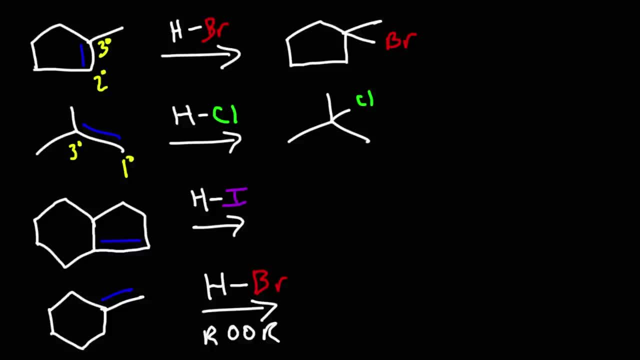 For the next example: where will the iodine go? Will it go on this carbon or on this one? So this carbon here is secondary. It's connected to two other carbons. This one here is tertiary because it's attached to three different carbon atoms. 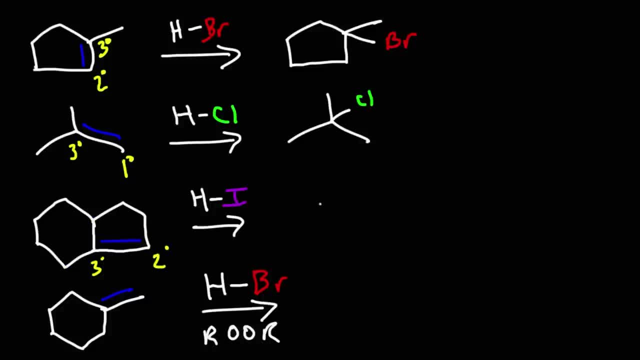 So this reaction is regioselective. It's going to proceed with more carbon decomposition. So the iodine atom is going to be added to the tertiary carbon. Now, once we add it to this carbon, will it be chiral? 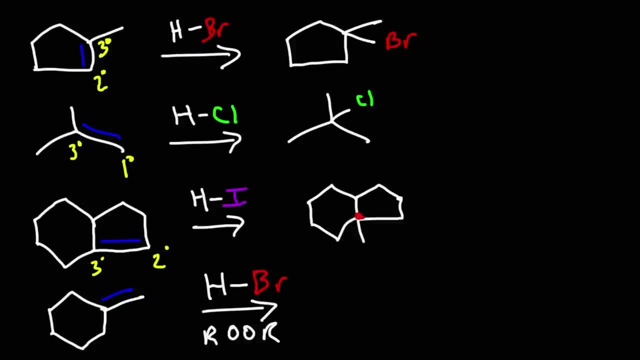 Is this carbon atom here, chiral, This carbon atom, would you say? it has four different groups. That's the question. Okay, I would say yeah, Once we place, Let me put the iodine atom here- Once we put it here, we're going to have a chiral center. 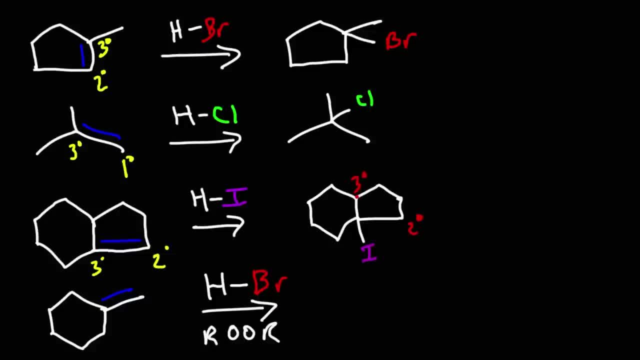 This carbon is secondary. It's different from this carbon, which is tertiary and this one is secondary. These two secondary carbons are not identical. The one on the left is on a sixth carbon ring, The other one on the right is in a five carbon ring, and so they're different. 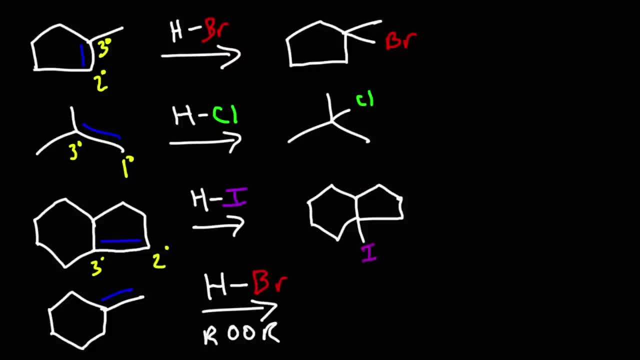 So we have a carbon with four different groups, so we have a chiral center, which means we need to show stereochemistry. The iodine atom could be on the wedge or it can be on the dash, so we need to show both because we get two different products. 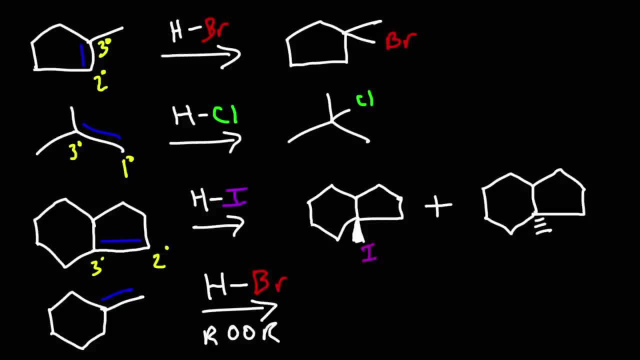 Okay, Okay, Okay. So these two are on the same越 sugar, these two are on the same hexagonal ring. This is a positivelymonsidide heroine. Okay. So where do we start? It starts off in the twelfth chemical element, which just takes oxygen energy. 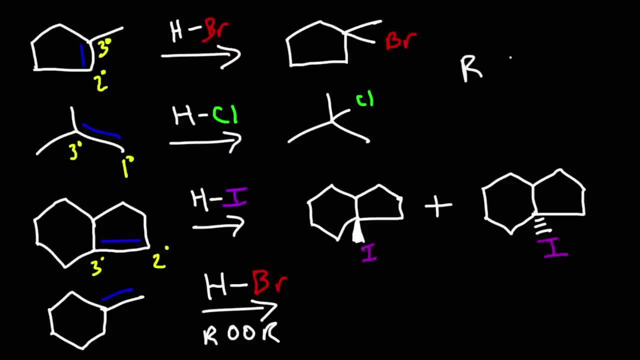 So if we take a bit of oxygen energy, this is just like just as bright as this, but we only need to add one good group here. So there are two of these, And that's because this is totally plus Cu2OH6.. 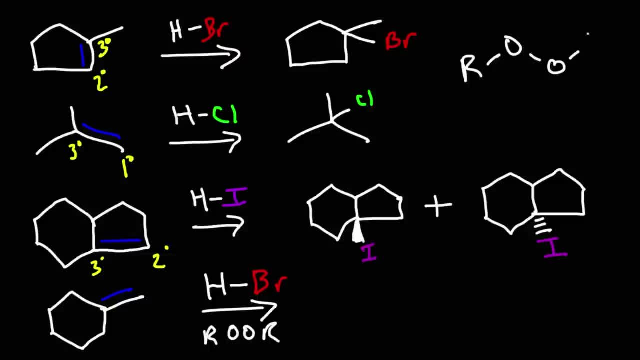 And I think another way in which we're going to do this is that this wasibo должна には sor ث, Whether this solbonit, which is thevanol. Let's see if we were to put a number in here, Okay. 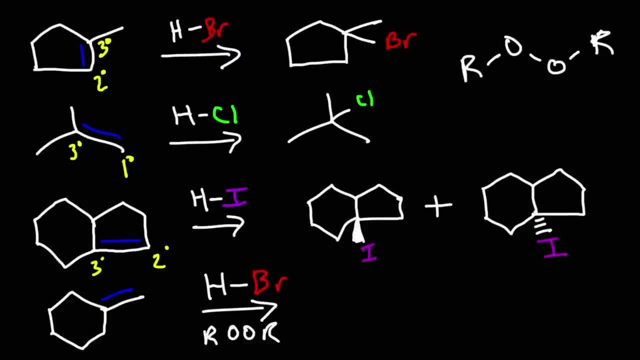 So this is the range between those two. how about this one? Okay, So here this will be a little bit perfect scale from this catalyst. It reacts in a similar way as hydrogen peroxide, So if you were to see ROOR or H2O2, they will have the same effect when used in connection with HBr. 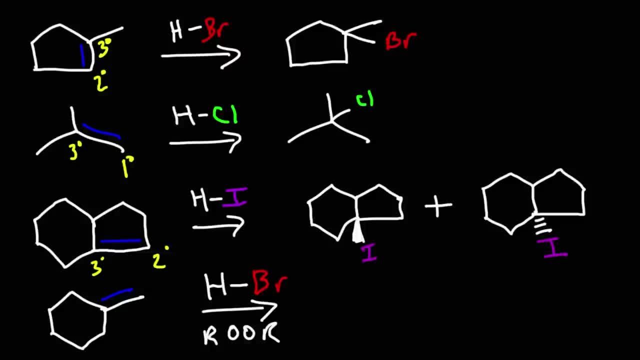 So first we need to determine which carbon atom, the bromine atom, is going to go on. This carbon is primary, this one is tertiary. When you have HBr in the presence of a peroxide, we know the reaction is going to proceed with anti-mercarbonic carbon addition. 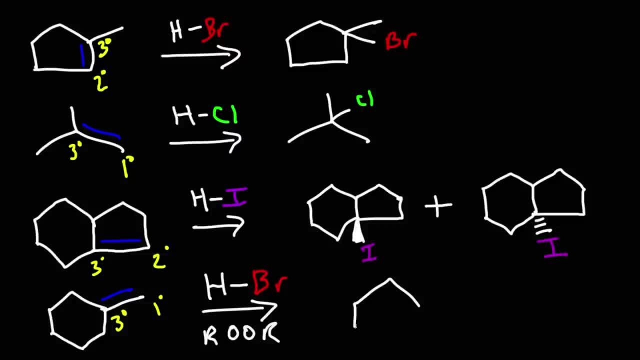 So the bromine atom is going to go on the least substituted carbon atom of the double bond. So that is, it's going to go on a primary carbon. So this is going to be the major product of the reaction. This carbon is not chiral, so we don't need to indicate stereochemistry for this example. 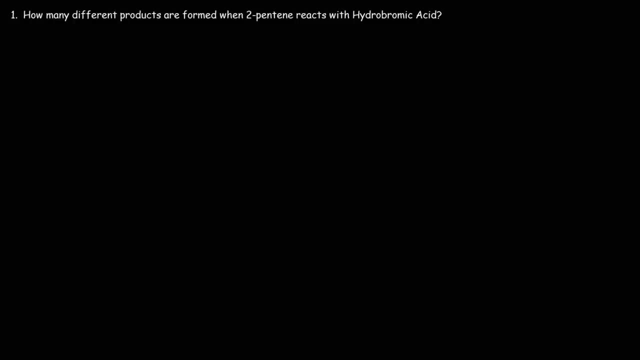 Let's work on this example problem: How many different products are formed when 2-pentene reacts with HBr? Well, let's find out. So first let's draw 2-pentene. So we're going to draw pentane, which is a 5-carbon chain. 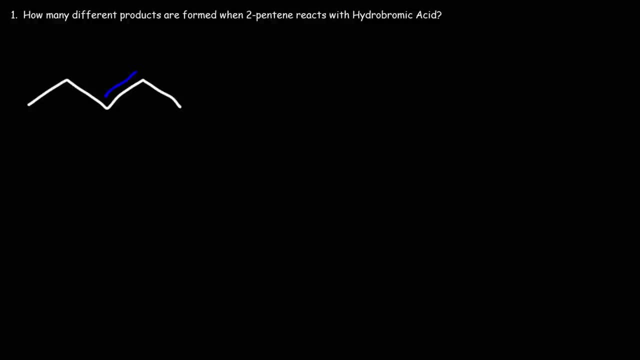 And then we're going to put the double bond between carbons 2 and 3. So this would be 2-pentene if we count it this way. So now let's react it with HBr. This reaction is not VGL selective, because both atoms, both carbon atoms, across the double bond have the same substitution. 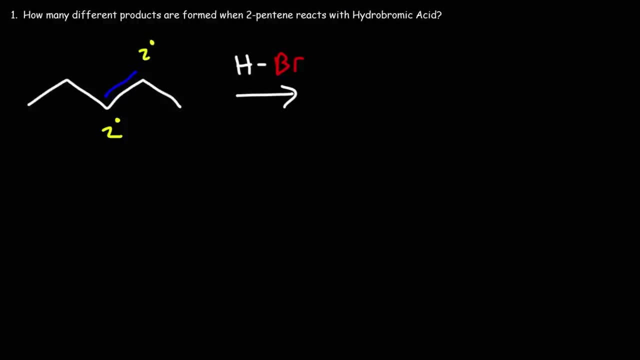 They're both secondary, So the bromine atom can go on either one. Thus we're going to get an equal mixture of 3-bromine atoms and 1-hBr. So we're going to get an equal mixture of 2-bromine atoms and 1-hBr. 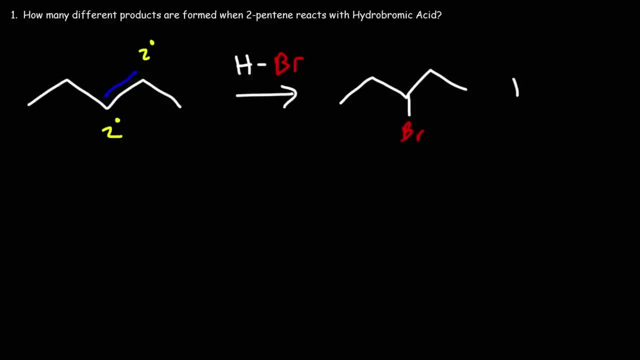 pentane and 2-bermopentane, so we're going to get these two different products now. the goal of this problem is to determine the number of different products, so we need to take into account stereochemistry. this carbon atom is not chiral because we have two identical ether groups, so 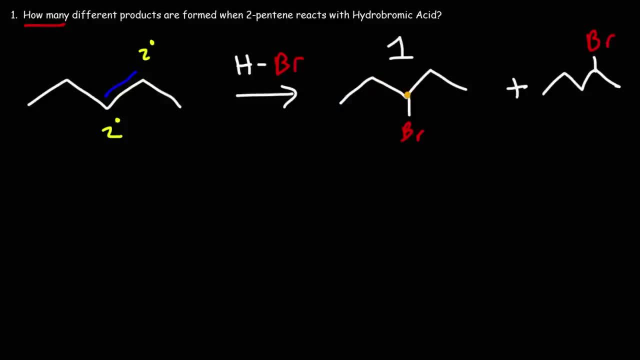 therefore, we only get one product of this type. now, 2-bermopentane does contain a chiral center. this carbon has four different groups: it has a bromine atom, it has a hydrogen, it has a methyl and it has a propyl group. so this is a chiral center, which means we can get two different. 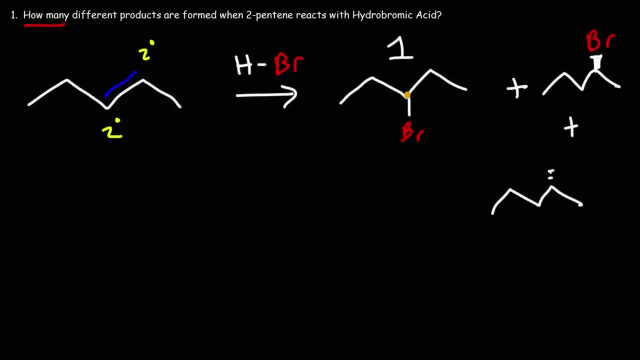 stereoisomers of 2-bermopropane. so, taking stereoisomers into account, we get a total of three different products. so that's it for this problem. number two draw the major product formed from the reaction between 3-methyl 1-pentene and the hydro bromic acid. so let's begin by 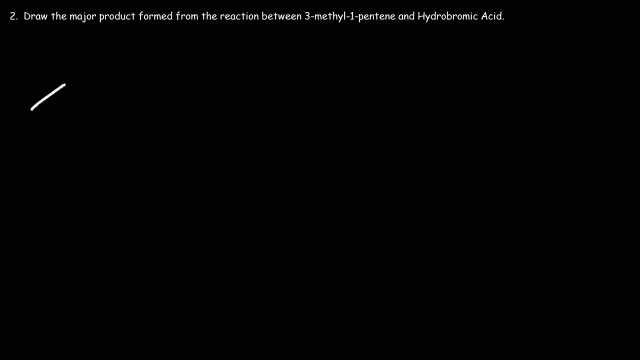 drawing three methyl, one pentene. so this is pentane and we're gonna put a double bond between that and 3-methyl 1-pentene. and that is important when you give with氧iones in the articles Á0ure yásか. 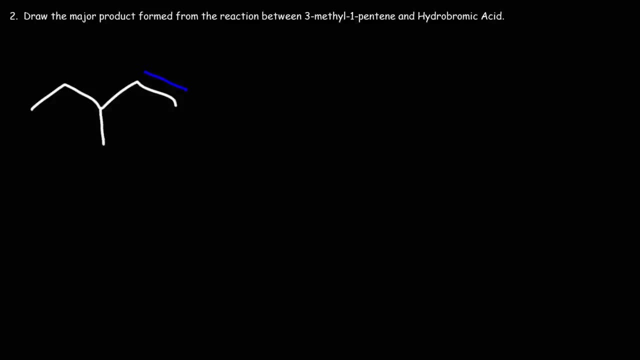 carbons 1 and 2.. And then we have a methyl on carbon 3.. Now let's react this with hydrobromic acid, HBr. Now you might be thinking: okay, we need to break the double bond and we need to put the bromine atom on the more substituted. 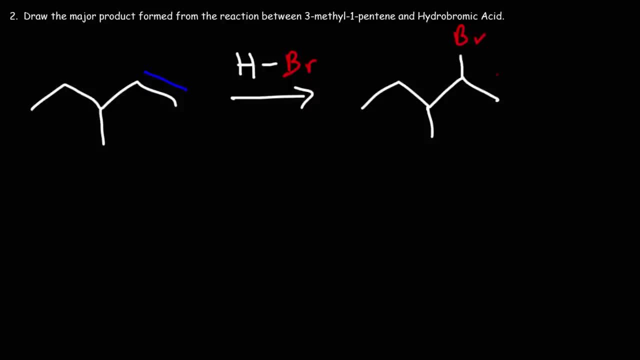 secondary carbon, And if you're thinking that way, that's a good start. But it turns out that this is not going to be the answer, Even though we know this reaction will proceed with Makarov-Lakhov regiochemistry, and it's preferable to. 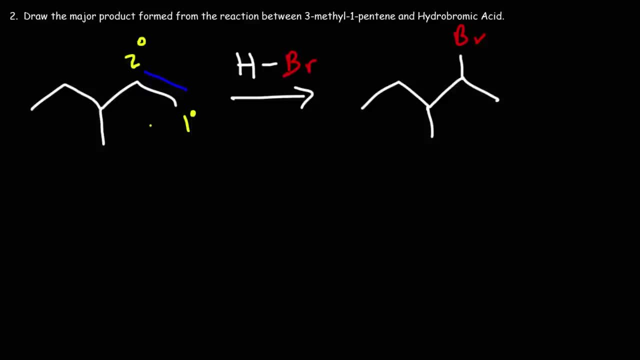 put the bromine on the secondary carbon as opposed to primary carbon. we do have a tertiary carbon, adjacent to the alkene, or to the double bond rather, And so what we're going to get is a carbocation rearrangement. Thus, in order to get the 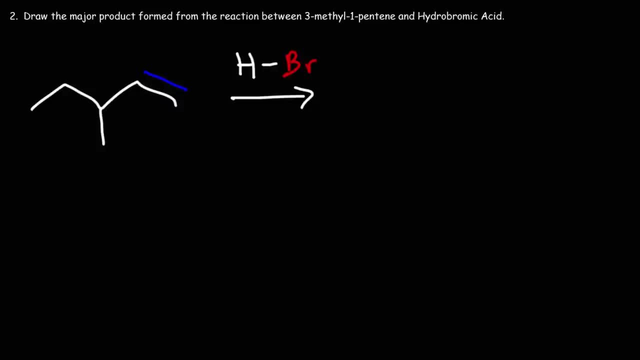 right answer. we need to show the mechanism for this problem. The nucleophilic double bond is going to react with HBr, The pi bond is going to break and we're going to form a new sigma bond between the primary carbon and the hydrogen. So this is going to create initially a secondary carbocation. 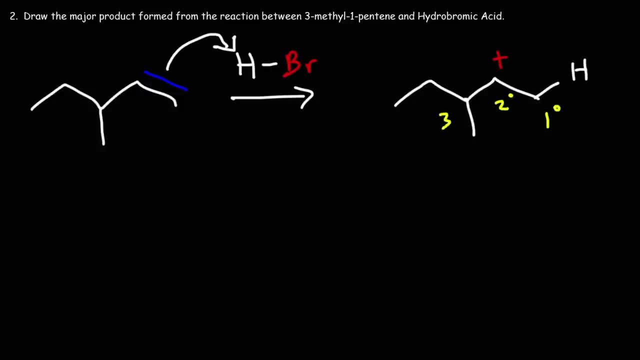 intermediate. Now, whenever you have a secondary carbocation adjacent to a tertiary carbon, where are you going to get the right answer? You're going to get the to get is a hydride shift. the hydrogen on the tertiary carbon is going to shift towards the secondary carbon as it leaves the tertiary carbon. it's going to. 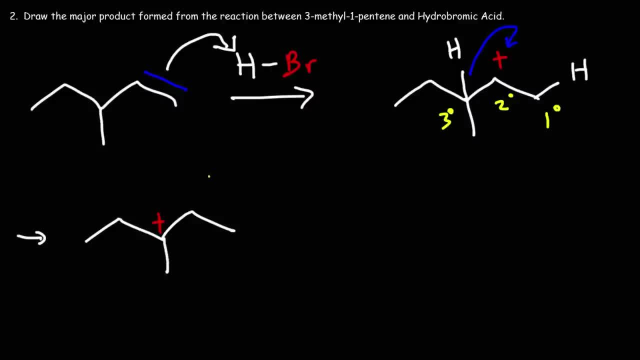 leave behind a positive charge, and so now we have a more stable tertiary carbocation intermediate. now, once this intermediate forms, the bromide ion is going to react with it, and so this is going to be a major product. 3-bromo-3-methylpentane. 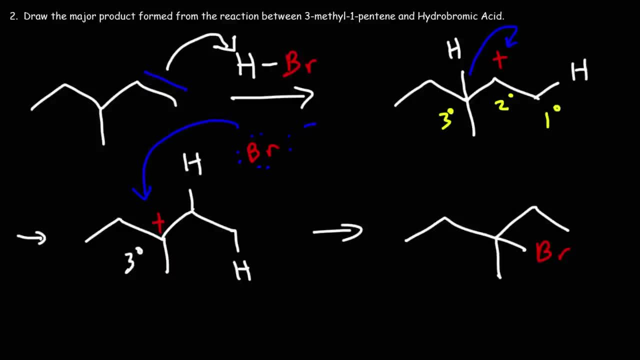 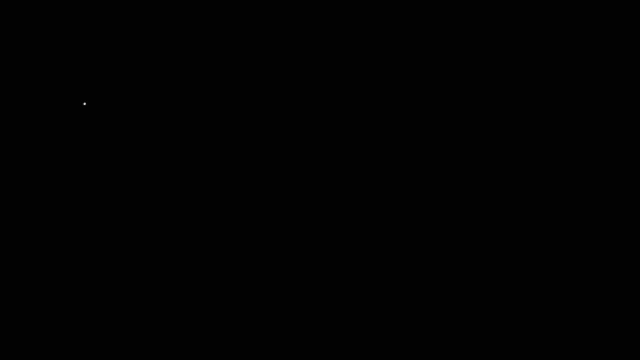 now, these two ethyl groups are identical, so stereochemistry is not relevant in the product of this reaction. so this is going to be the answer. now I want to take a minute to talk about the textbook definition of Mokarmdokov's rule, because we described it in terms of carbon atoms as opposed to in terms of 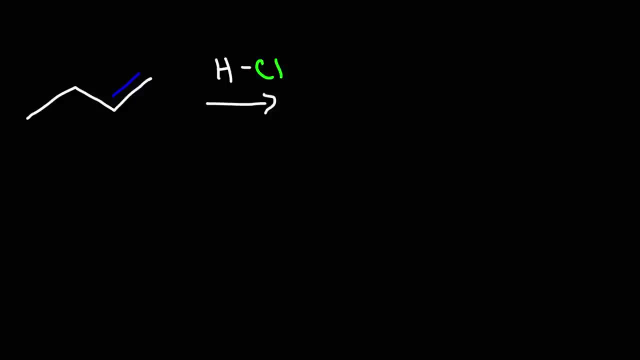 hydrogen atoms. in fact, the textbook definition of Mokarmdokov's rule is that the H plus in HCl or HBr that's going to go on the carbon with more hydrogen atoms. so in this case that's going to be the primary carbon. the primary carbon has two hydrogen atoms. the secondary carbon has: 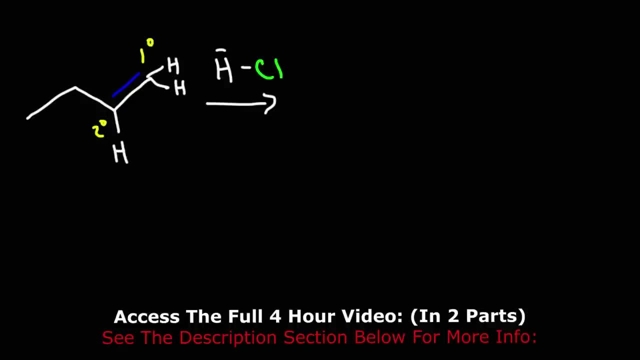 one. so according to Mokarmdokov's rule, this hydrogen is going to go on the carbon with more hydrogens. so once its double bond reacts with HDL, we're gonna put the hydrogen on the primary carbon and we'll get the plus charge on the secondary carbon. so that's a textbook definition of 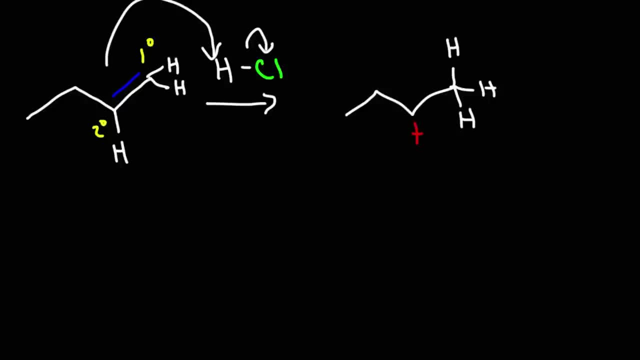 Mokarmdokov's rule, but the end result is that the chlorine is going to go on the more substituted carbon atom with a double bond. when taking a test, it's easier to view it in terms of the hydrogen. now the result is: this is going to go on the second bond and that is going to be above a minimum carbon atom. carbon amount played carbon: МосF1a- x2mmol. 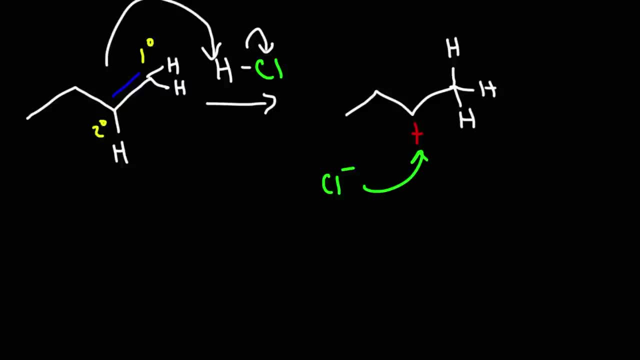 in terms of the chlorine content. so again, the experiment is going to be atense. そし view it in terms of carbon rather than hydrogen. It's easier to identify which carbon is more substituted across that double bond than counting the number of hydrogens. 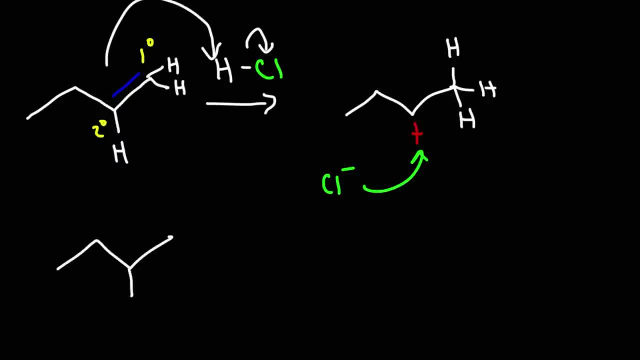 So I just want to make sure you're aware of that's how McCormick-Curve's rule is described. It's basically the addition of the H plus to the carbon atom. that's part of the double bond that has more hydrogen atoms. So now let's work on another example. 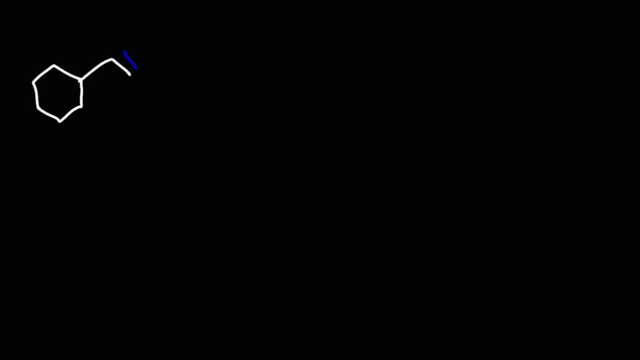 Let's react this alkene with one mole of hydrobromic acid, or we could say one equivalent of HBr and two equivalents or two moles of sodium iodide. What's going to be the product of this reaction? 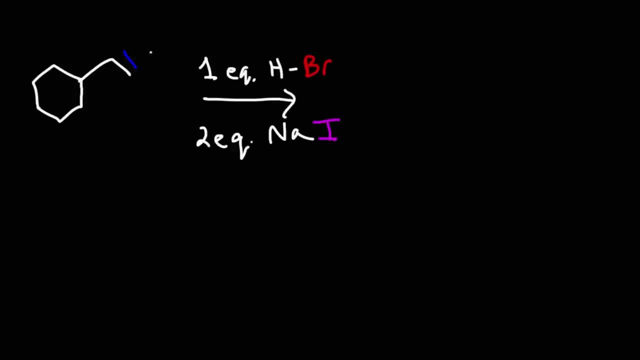 Feel free to work on this example. So the first thing that's going to happen is the alkene is going to react with hydrobromic acid According to McCormick-Curve's rule, the hydrogen. it's going to go on a primary carbon. 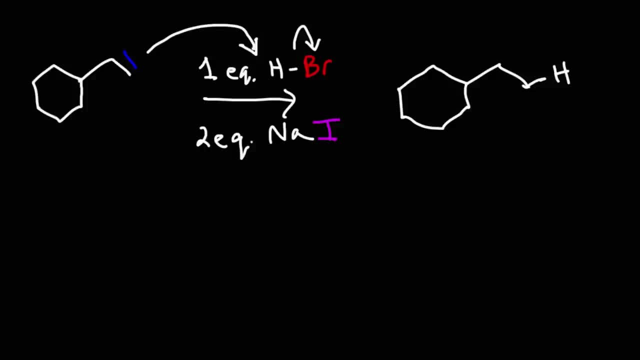 because that carbon has the most number of hydrogen atoms across the double bond And initially we're going to get a secondary carbocadine. Now that secondary carbocadine is adjacent to a tertiary carbon. So what's going to happen next is a hydride shift. 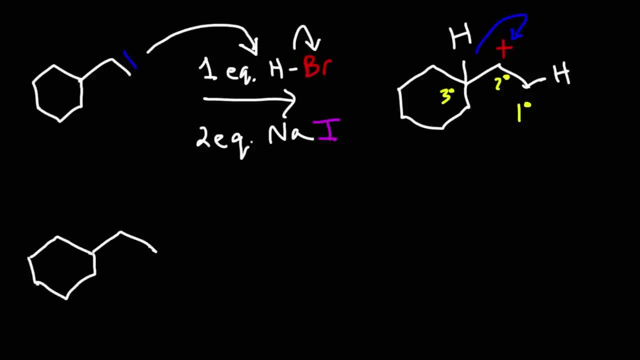 So now we're going to get a more stable tertiary carbon, So we're going to get a more stable tertiary carbocadine intermediate. Now what's going to happen here? We're going to get two different products. One possible product that we can get is that the bromide ion could react with the carbocadine. 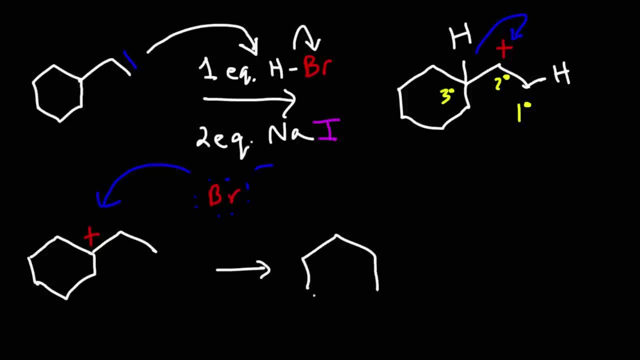 If that happens, we're going to get this product. Now we also have iodide in a solution, So iodide could also react with the carbocadine. So in this example problem we're going to get a mixture of products. 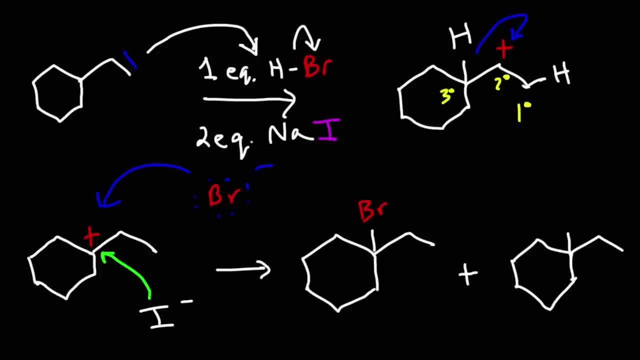 The question is which one is going to be the major product. The only way to answer that is to look at the concentration. The concentration of iodide is greater than the concentration of bromide because in the beginning we were told that we have two equivalents of sodium iodide and only one equivalent of HBr. 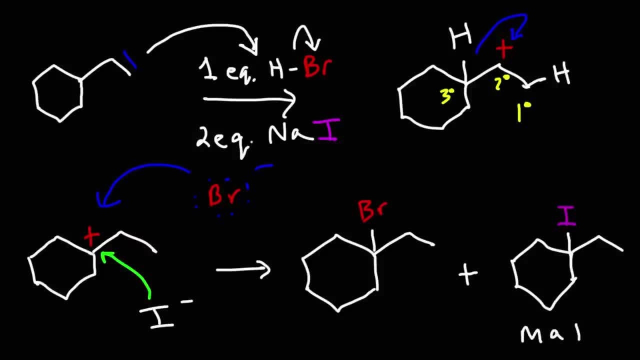 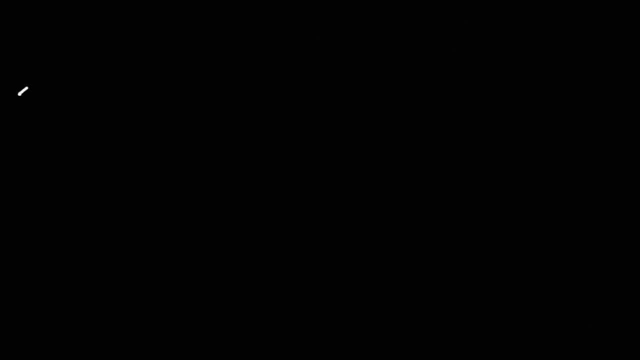 Therefore, based on concentration, this is going to be the major product and this will be the minor product. Now let's consider some other reactions, So starting with 3.5.. So this is going to be the major product And this will be the minor product. Now let's consider some other reactions, So starting with 3.5. 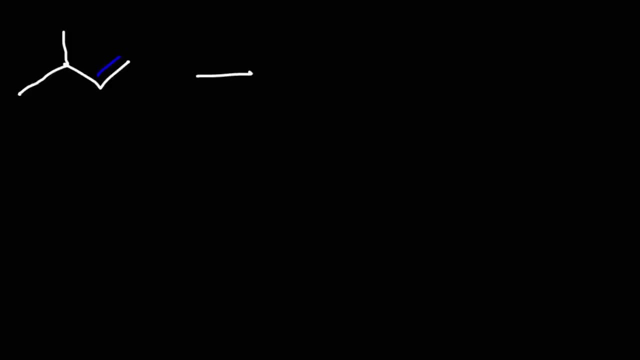 Let's consider some other reactions. Now, let's consider some other reactions, And this will be the minor product. now Lets react that particular alkene with the H3O plus the hydronium ion. We're also going to react it with. 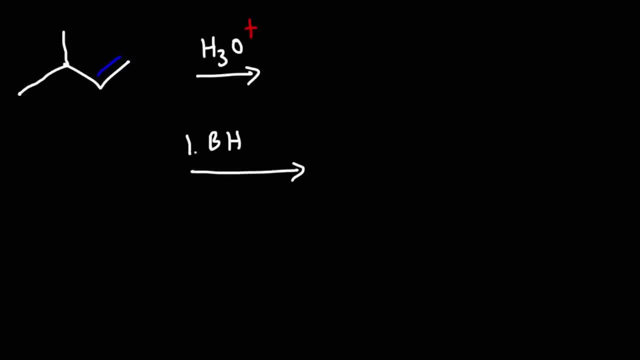 This is a separate reaction, by the way, But we're also going to react it with BH3 boron. I mean not boron, but Borain with THF and the second step. We're going to react it with BH3 boron. I mean not boran, but borain with THF and the second step. 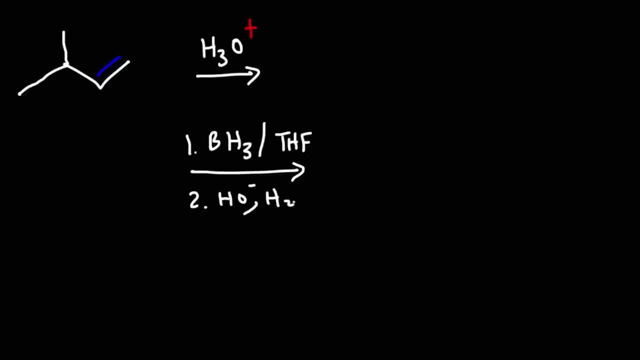 We're going to react it with? We're going to react it with Hydroxide, hydrogen peroxide and water. We take that as a single ingredient. we then add in our concentration And then for a third reaction, in the first step we're going to have mercury acetate with water, followed by sodium borohydride, NABH4.. So what's going to happen if we mix this particular alkene with H3O plus? When H3O plus reacts with an alkene, it's going to form a carbocation intermediate. As a result, it's subject to rearrangement. 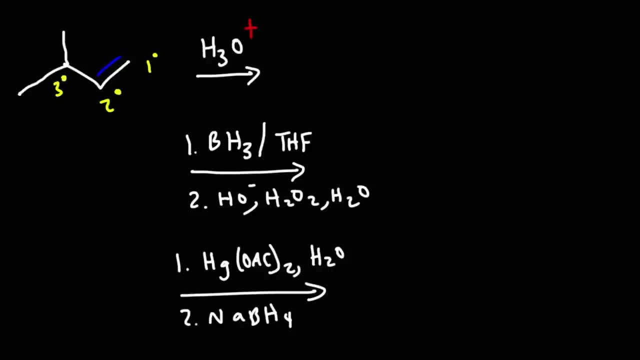 Now this particular alkene has the ability to rearrange, because we have a tertiary carbon adjacent to a secondary carbon. that's part of the alkene. So we're going to get a hydride shift and the end result of this reaction is going to be NABH4. 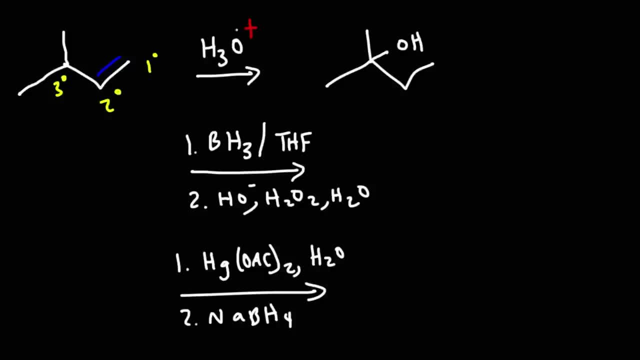 So we're going to get a hydride shift and the end result of this reaction is going to be a tertiary alcohol. So this reaction proceeds with marcarbonic carbon addition, but it's subject to rearrangements. The OH is going to go on, typically the most substituted carbon atom, that's adjacent to a double bond. 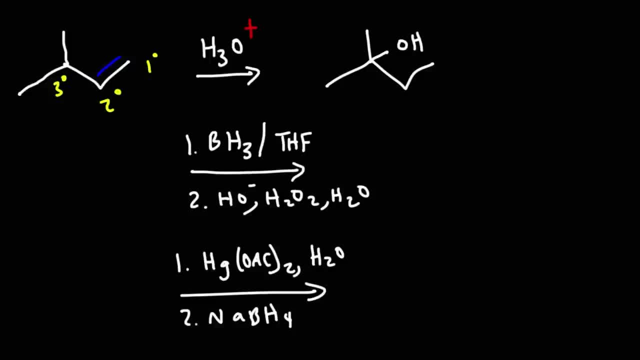 Now for this reaction: hydroboration oxidation. this reaction proceeds with anti-marcarbonic carbon regiochemistry. The OH is going to go on the least substituted carbon atom, In this case the primary carbon. For the next reaction, we have oxymercuration, demercuration. 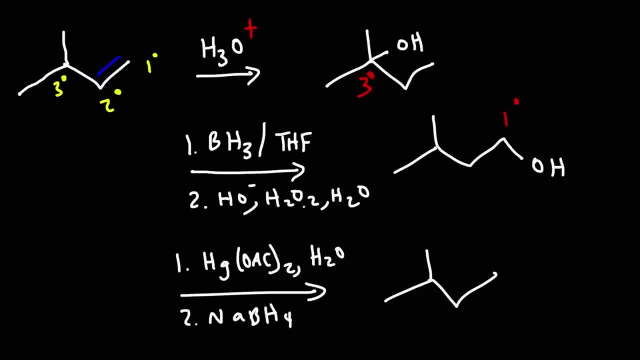 The hydroxyl group is going to go on the secondary carbon. It's going to go on the most substituted carbon of the double bond. So this reaction proceeds with marcarbonic carbon regiochemistry. However, it does not rearrange. So here we're going to get a tertiary carbon atom. 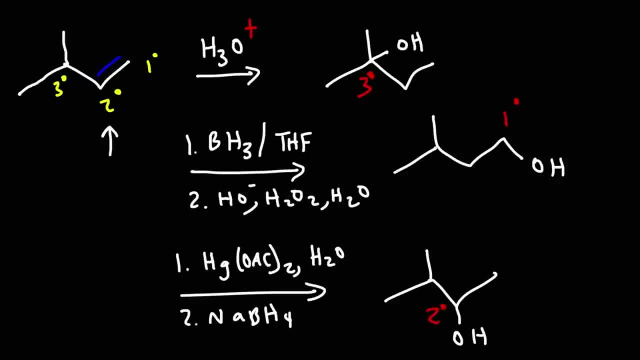 So here we're going to get a tertiary carbon atom. So here we're going to get a tertiary carbon atom, secondary alcohol instead of a tertiary alcohol. So make sure you know the differences between these three reactions. So this one proceeds with antimicrobial-carbohydrate chemistry. The OH is going to go on the least. 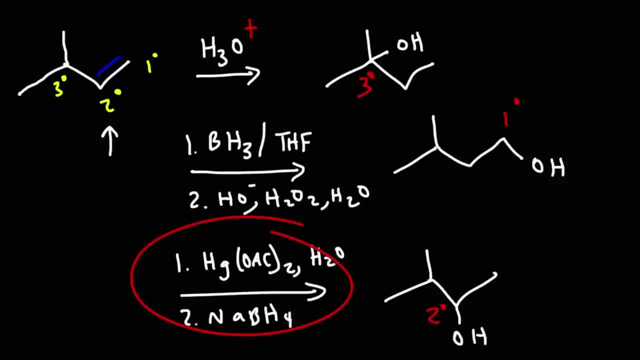 substituted carbon of the double bond. This one proceeds with carbohydrate chemistry. The OH is going to go on the most substituted carbon atom of the double bond, And for this one it's susceptible to rearrangements. So it really depends on the structure of the alkene. 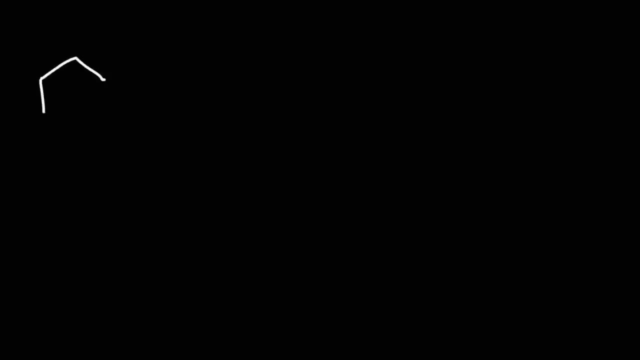 So let's say we have this particular alkene And we're going to react it with water and sulfuric acid. What's going to be the major product of this reaction? The first thing you need to realize is that sulfuric acid is a strong acid When 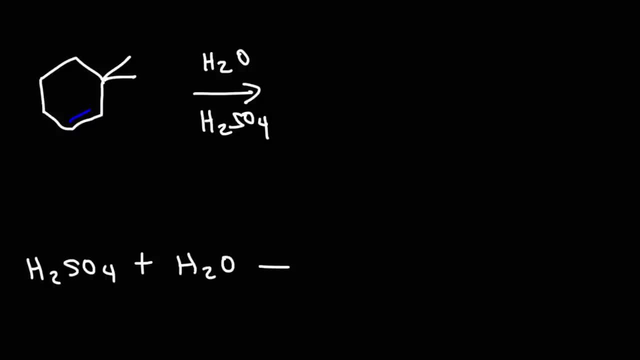 it reacts with water. water is going to act as a weak base, So sulfuric acid is going to donate a proton to water, creating H3O plus and the bisulfate ion. So this reaction produces H3O plus. So mixing an alkene with water and sulfuric acid. 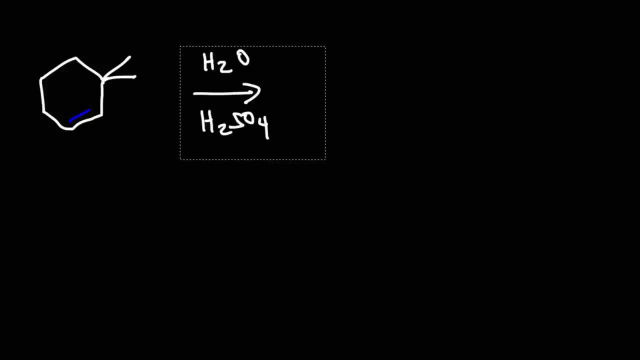 water and sulfuric acid is equivalent to react in it with H3O plus Now. the first thing that's going to happen is the alkane is going to react with a hydrogen in H3O plus Now here's a question for you. 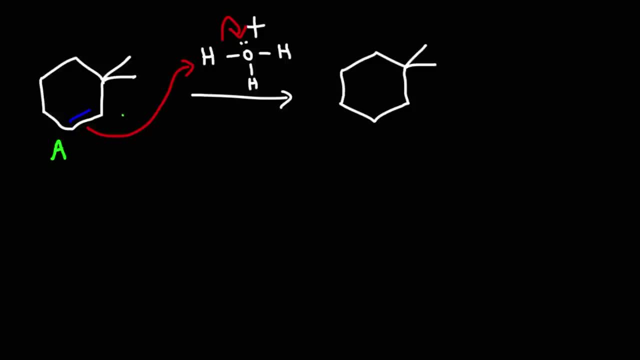 On which carbon atom will the hydrogen go? Will it go on carbon A or carbon B? Both carbon A and carbon B. they're equally substituted. they're both secondary carbons, So which one will it go on? In this case, Markovnikov's rule won't help us. 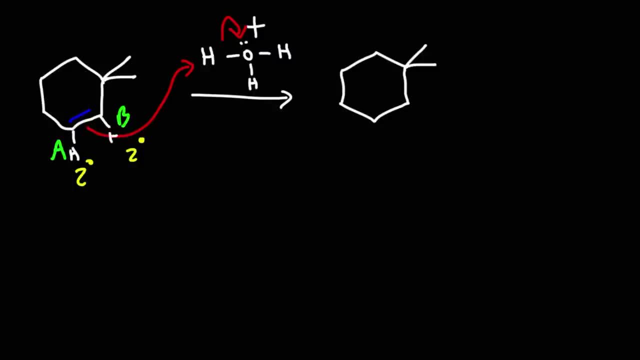 Because they're both secondary, they both have the same number of hydrogen atoms. Okay, But the hydrogen is going to go on carbon A. The reason for that is the plus charge wants to be next to the quaternary carbon, Because a methyl shift can occur, giving us a more stable carbocation intermediate. 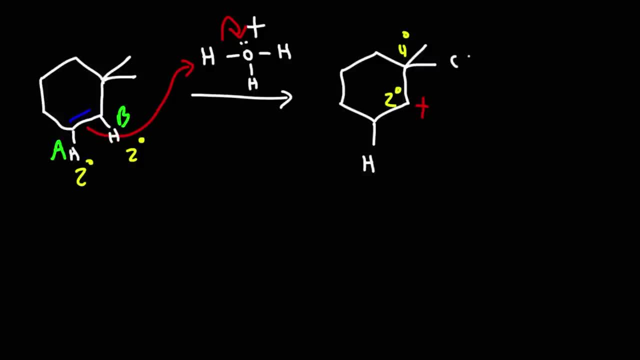 Right now we have a secondary carbocation intermediate, But once we move the methyl we can get a tertiary carbocation intermediate. The driving force for these carbocation rearrangements is the H3O plus. The H3O plus is going to be next to the quaternary carbon because a methyl shift can occur, giving 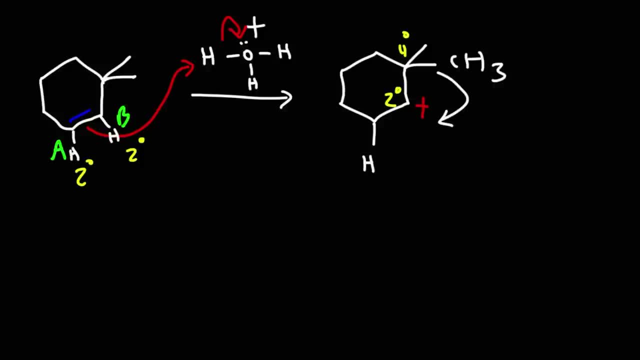 us a more stable carbocation intermediate. Okay, So the first part of the chain of changes is stability. The carbocation will rearrange in such a way until it finds the most stable form that it can acquire, And so we're going to get this methyl shift. 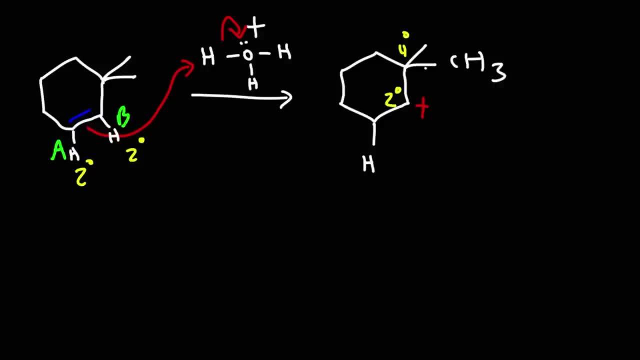 So this arrow is going to start from this bond, the two electrons in this bond, and it's going to point towards the carbocation And so the entire carbon-carbon structure. Okay, going to change. My drawings are terrible. I need to do this better. 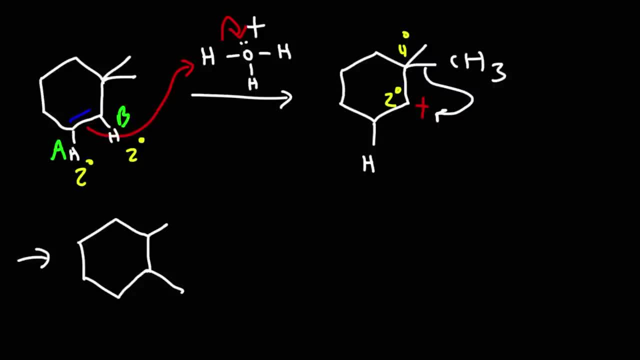 So now this carbon atom? it lost a bond. That's where the plus charge is going to be. So right now, what we have is a tertiary carbocation intermediate. We went from a secondary carbocation to a tertiary carbocation, And now at this: 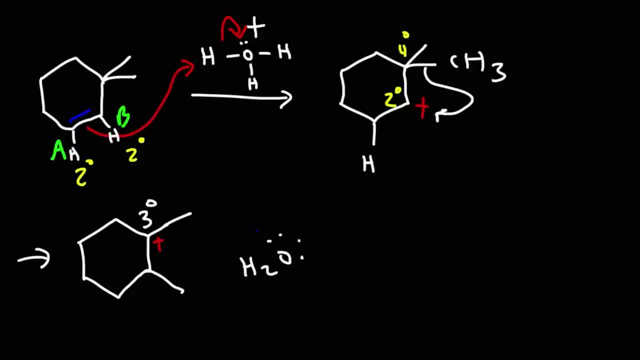 point. water can react with the tertiary carbocation, And what we're going to get at this point is something known as an axonium ion. And then we're going to use another water molecule to remove one of the hydrogens, And this will give us an alcohol. 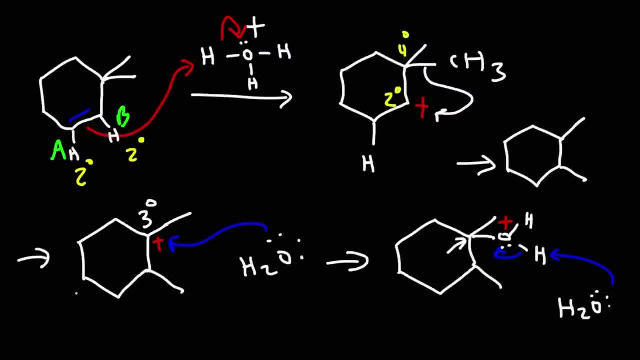 Now this carbon- here it's a chiral carbon, And water could attack from either side, So we can get a mixture of isomers here, But we're not going to worry about it too much, So I'm just going to put: OH, Just know that we can. 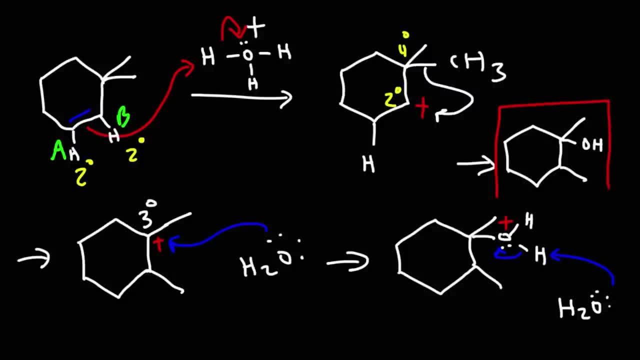 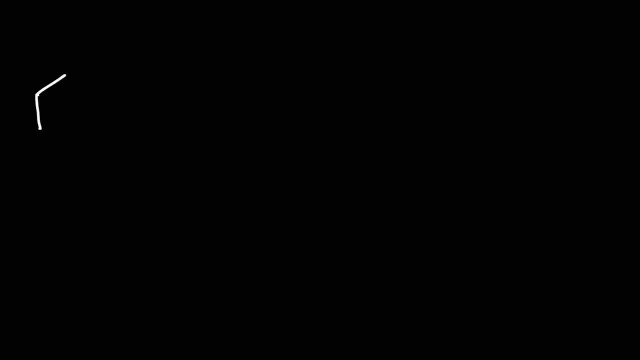 get a mixture of stereoisomers, So that's going to be the major product for this particular reaction. Go ahead and try this one. What's going to be the major product if we react this alkene with dilute sulfuric acid in methanol, So methanol is a solvent in this reaction. 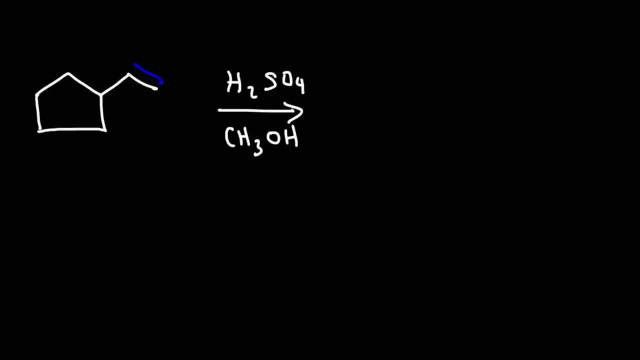 What's going to happen here? Sulfuric acid can give away a proton, And that's what's going to happen: The alkene is going to acquire a proton. Now, this proton can come directly from sulfuric acid or it can come from a protonated solvent molecule. So, just as 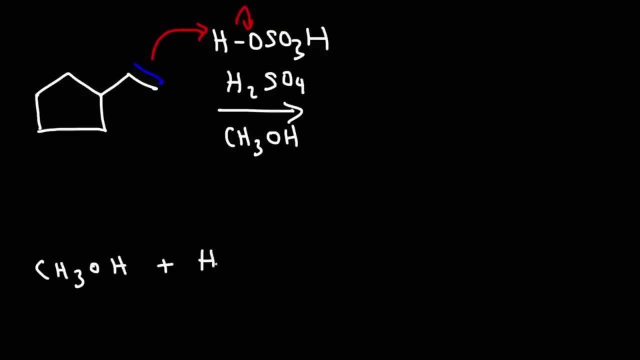 water can react with sulfuric acid. it can come from a protonated solvent molecule, acid. methanol can also react with sulfuric acid And we can get the conjugate acid of methanol and HSO4. So this alkene can acquire a proton from. 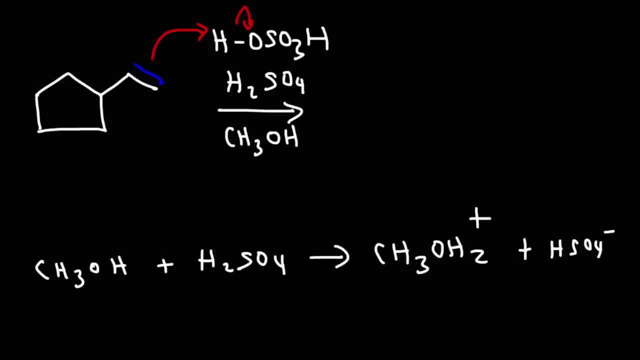 that species as well. So there's more than one way to show the mechanism. just keep that in mind. So, regardless of where the alkene gets the proton, we're going to end up initially with the secondary carbocation. Now, what do you think is? 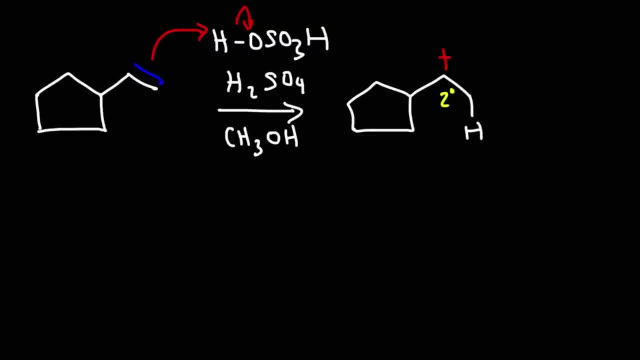 going to happen next? Well, we do have a tertiary carbon here, so we could get a hydride shift, But notice that we have a five carbon ring Whenever there's a potential for a rearrangement. if you have a five carbon ring, there's a. 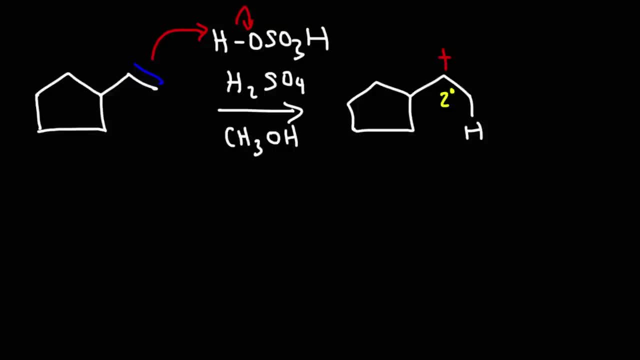 possibility that you can get a ring expansion. A six carbon ring is more stable than the five carbon ring. A six carbon ring has less angle or ring strain. so that's what's going to happen here: we're going to get a ring expansion. 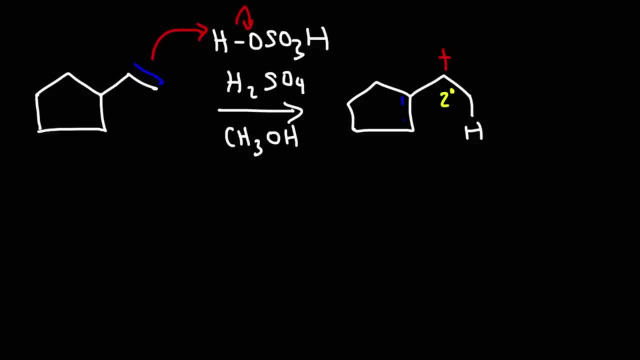 Let's call this carbon one, two, three, four and five. So the signal bond between carbons 1 and 5, that's going to break. Those electrons will be used to connect the secondary carbocation, which let's call it carbon 0. So the electrons between carbons 1 and 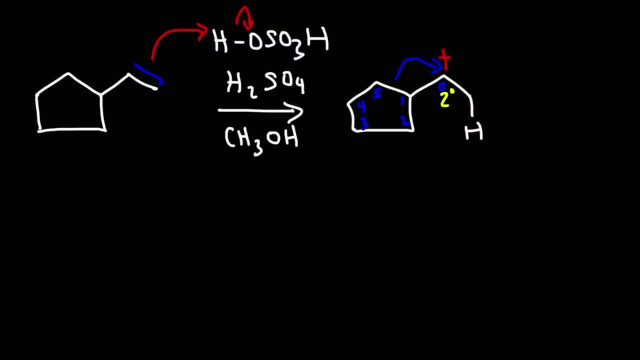 5 is going to connect carbon 0 and carbon 5.. And so we're going to get a 6-carbon ring which is going to look like this: Now let's call this carbon 5, carbon 0,, 1,, 2,, 3, 4.. Carbon 0 has a method group attached to it. 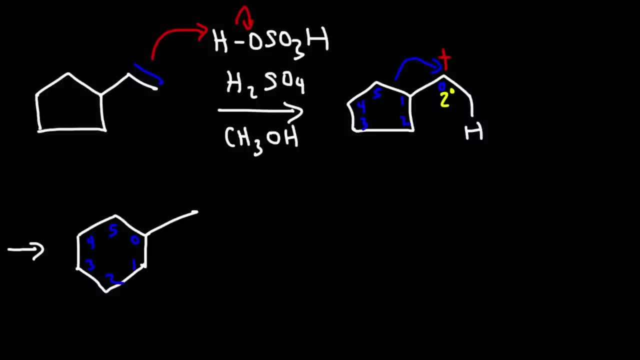 Now which carbon atom has the plus charge? Is it carbon 0,, 1, or 5?? So we lost the bond between 1 and 5, but we formed a new one between 0 and 5.. So carbon Carbon 1 lost a bond and it didn't get anything back. 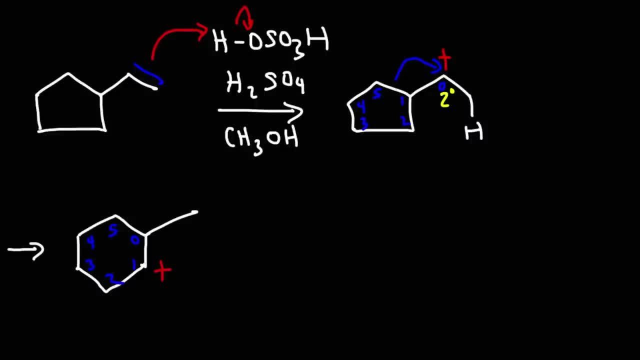 Thus carbon 1 has the plus charge. So right now what we have is a secondary carbocation. So far the stability has been improved Here. we had a secondary carbocation with a 5-carbon ring. Now we have a secondary carbocation with a 6-carbon ring. 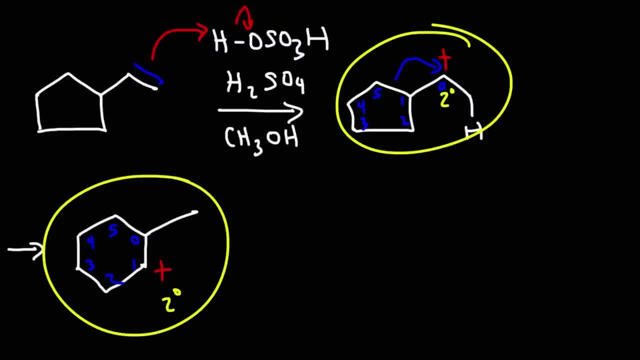 So we have a structure that's more stable than the previous one, But we're not done. Another rearrangement can occur because we have a tertiary carbon adjacent to a secondary carbocation intermediate, So a hydride shift is going to be the next thing that's about to happen. 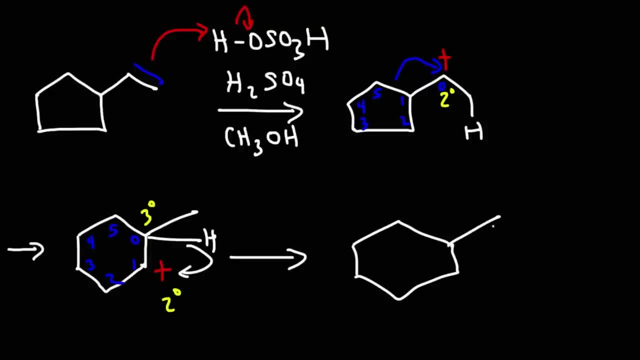 So after this hydride shift, we're going to have a 6-carbon ring with a tertiary carbocation intermediate, And we really don't need to show the hydrogen here. So now the next thing that's going to happen is methanol. 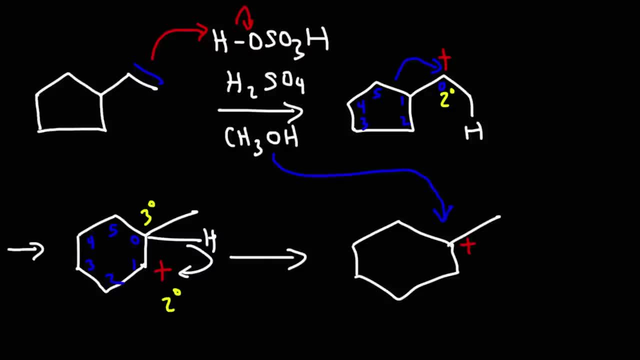 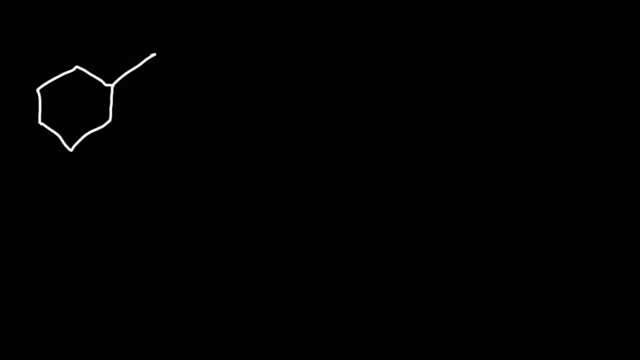 It's going to react with a carbocation intermediate, And so we're going to get an oxygen with a plus charge and 3 bonds. Now another methanol molecule is going to react with an oxygen, And so we're going to have a oxygen with a plus charge and 3 bonds. 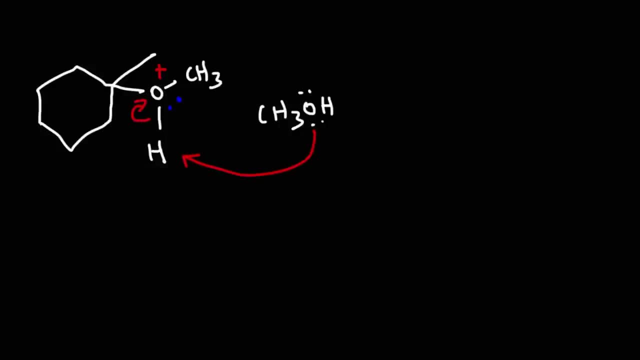 And so we're going to get another oxygen with a plus charge and 3 bonds is going to remove this hydrogen and the end result of this reaction is an ether. So that's what happens when you react an alcohol with an alkene: you're going to get an ether. 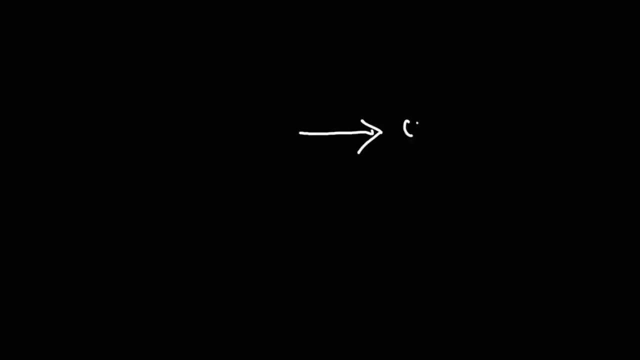 So now let's work on this synthesis problem. Consider the following ether- actually, let's make this a C- What alkene and what alcohol can you use to make this particular ether? Feel free to pause the video If you want to. So, in order to determine the type of alcohol and alkene that you need, you need to know. 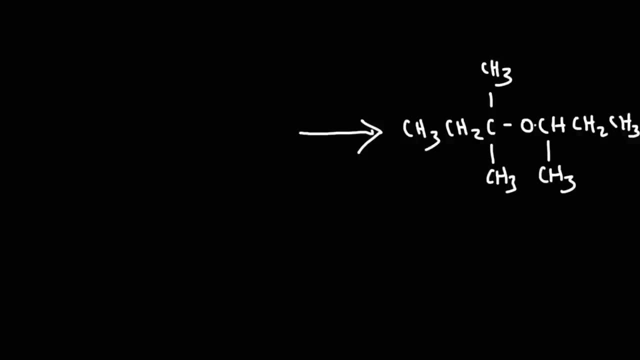 where to split the molecule and you want to split it basically at the carbon oxygen bond. So we could split it here or here, but let's focus on splitting it here. So this part has the oxygen. That's where the alcohol is going to be. 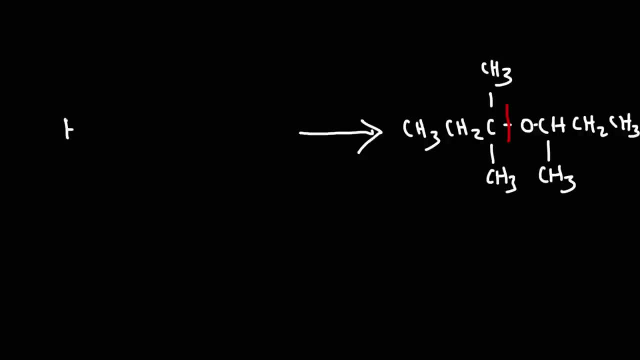 So I'm going to redraw the right side first. That is this part. I'm going to draw everything that I see here. I'm just going to add a hydrogen to the oxygen, So let me put that in a different color. So here's the hydrogen and then the oxygen, and I'm going to draw exactly what I have. 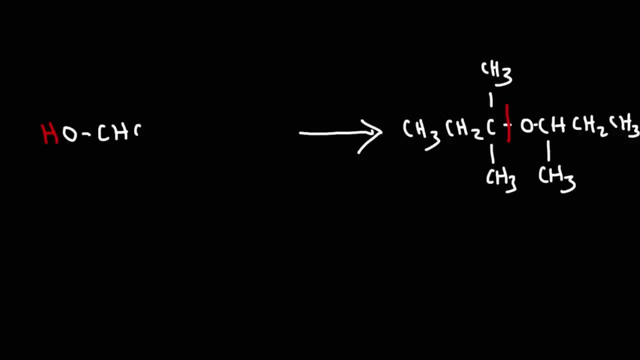 here, Okay, Okay. Now the other part is going to be the alkene, and I could put the double bond either here, here or here, So let's put it here. In order to put it here, I need to take off a hydrogen. 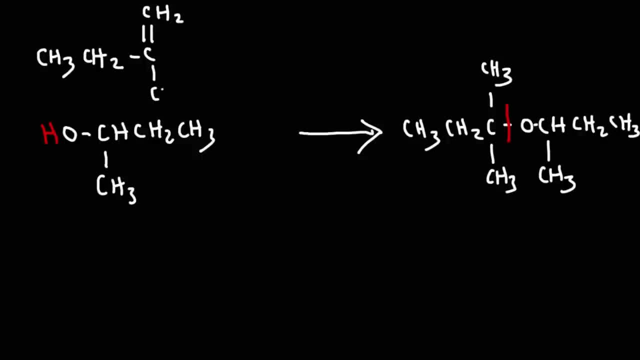 So it's going to be CH2 instead of CH3.. So this is one possible combination. If we react this alkene with this alcohol, we can make this particular ether. Now, if I were to put the double bond here, it would look like this: 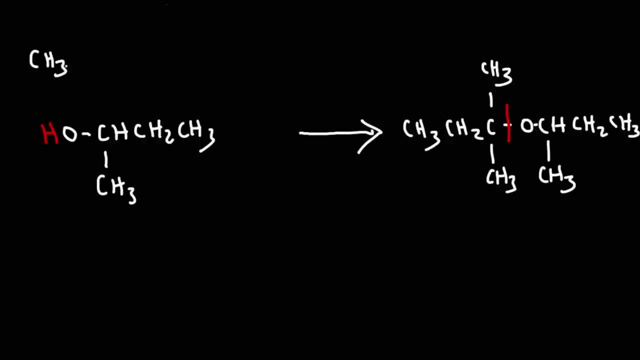 So I'm going to take a hydrogen from CH3.. From CH2.. So we're now going to have CH double bond C, and then that carbon has two methyl groups which I can just put here. So if I were to react this alkene with this alcohol, it would give me the same product. 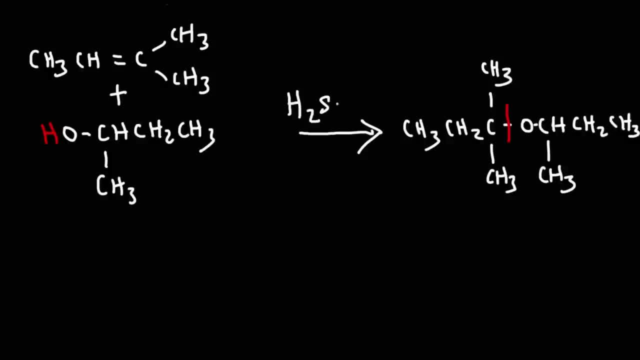 Now keep in mind we still need an acid catalyst to accelerate the reaction, So we would need H2SO4, dilute H2SO4, to get this reaction going. Now let's see what's going to happen, or what type of alkene and alcohol that we could use. 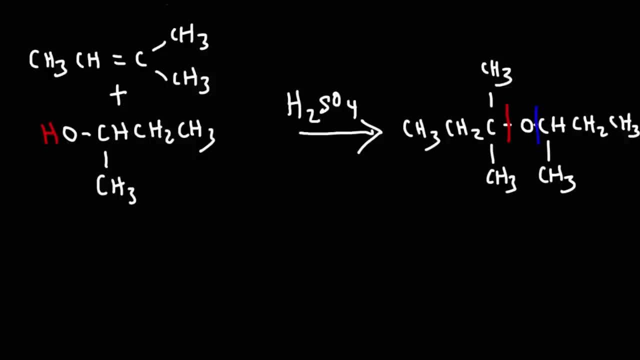 if we were to break the bond here, So if we were to break it there, this would be the alcohol that we're going to start with. So we're going to have CH3,, CH2, C, and then OH, And here we have two methyl groups. 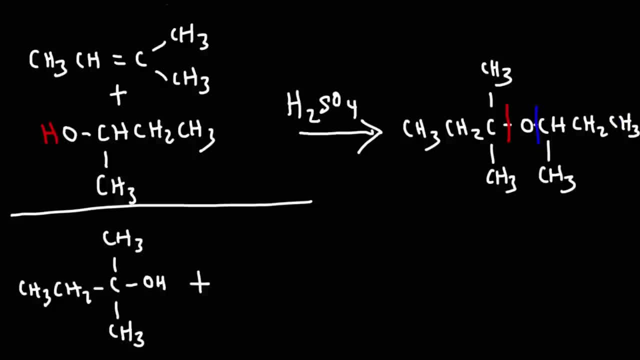 Now we can react this alcohol with two different alkenes. We could put the double bond between those two carbons or between those two carbons, So this is basically a four carbon chain that has no branches. If we put the double bond here, this is one butene. 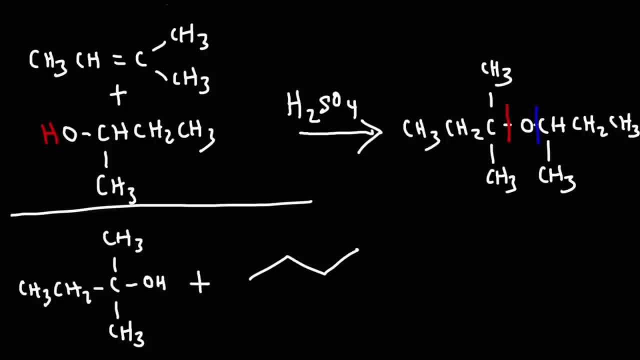 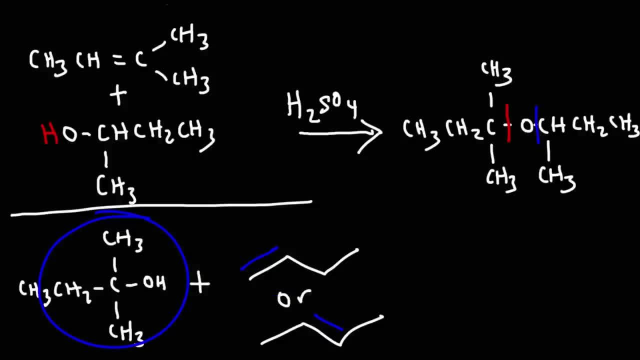 So this alcohol with one butene will give us the same product, or with two butene that will give us the same product as well. So far, we've considered four different combinations that could lead to this particular ether, And so that's how you could determine the initial parts. 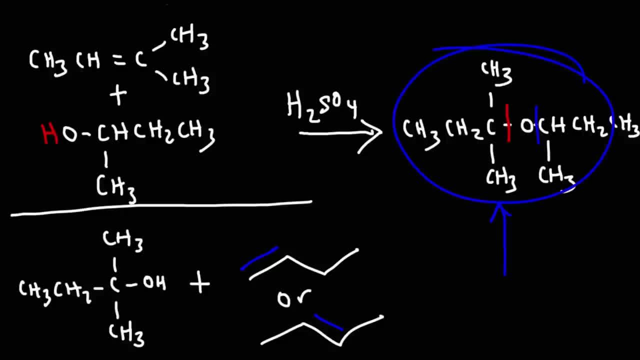 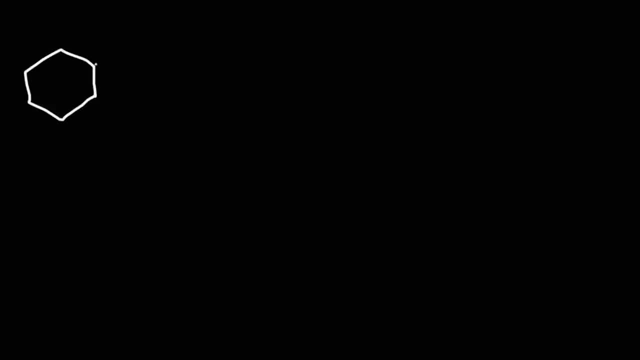 Now let's move on to our next problem. So let's say we have one methyl cyclohexene and we're going to react it with mercury acetate, with water, followed by sodium borohydride, And let's compare that to our next problem. So let's say we have one methyl cyclohexene and we're going to react it with mercury acetate, with water, followed by sodium borohydride, And let's compare that to another reaction. It's going to be a similar reaction. 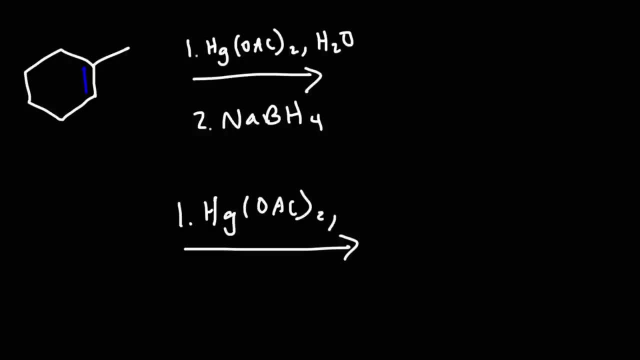 We're going to use mercury acetate again, but instead of using water we're going to use ethanol, CH3CH2OH, followed by sodium borohydride. So the first reaction is called oxymercuration-demercuration. The second reaction is alkoxymercuration-demercuration. 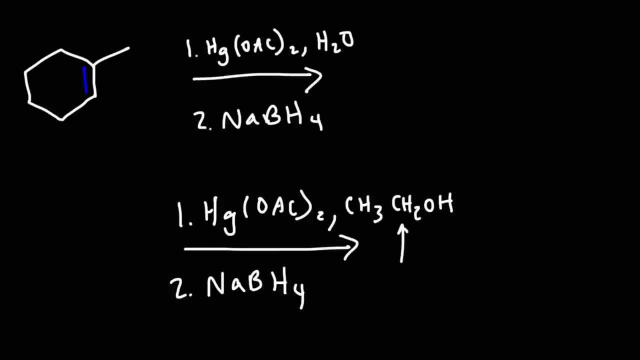 So the first reaction is oxymercuration-demercuration, because we're using an alcohol. Now we know this reaction proceeds with Markovnikov addition. So the OH group is going to go on the more substituted carbon atom of the double bond. 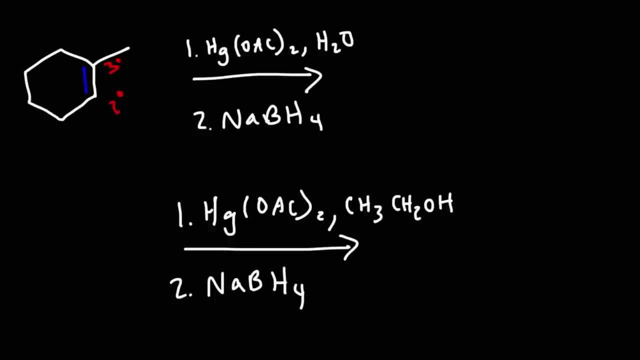 In this case it's going to be the tertiary carbon as opposed to the secondary carbon. So the end result for the oxymercuration-demercuration reaction is going to be alkyl, carbon-tox peroxide, which is the second carbon to go on. is that we're going to get an alcohol. The nucleophile is water. For the alkoxymercuration-demercuration reaction, the nucleophile is not water, it's an alcohol And whenever you react an alcohol within an alkene. 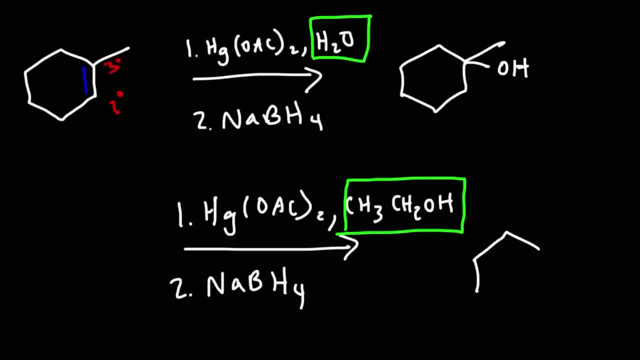 you're going to get an ether. So, instead of an OH group, we're going to get this product- It's basically what you see here- without this hydrogen. So we're just going to draw OCH2CH3.. So that's going to be the end result of this reaction. 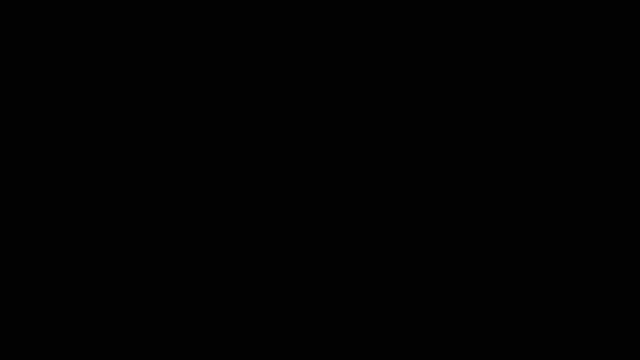 Now let's talk about the mechanism of the oxymercuration-demercuration reaction. So we're going to start with mercury acetate, which looks like this: Mercury acetate has two acetate groups and a lone pair, One of the acetate ions. 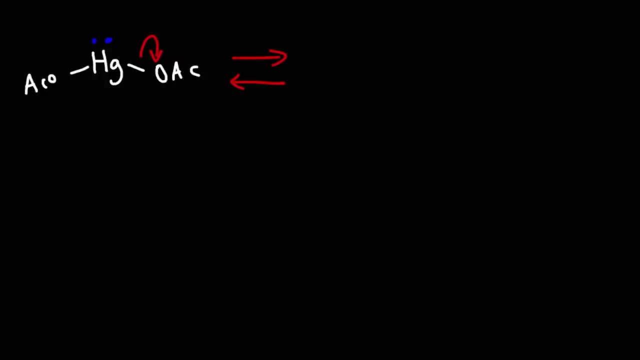 or one of the acetate groups can easily dissociate from mercury, And so we're going to get a mercuric cation which looks like this and a free acetate ion. Now, whenever you see OAC, basically this is acetate. 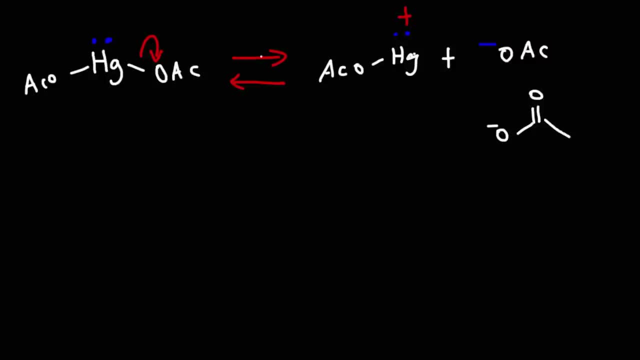 which looks like that. So this is reversible. The acetate can always rejoin with the mercuric ion to produce mercury acetate. So this process goes backwards and forwards. Now, once we form mercury acetate. now, once we form, 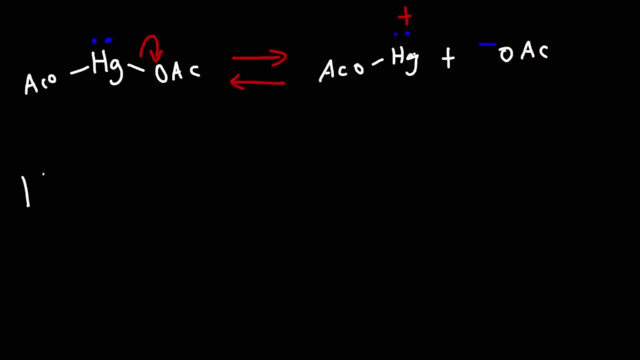 this mercuric cation. we can react it with an alkene. So mercury has a positive charge, Therefore it's an electrophile. The alkene is going to be the nucleophile. So we're going to draw the arrow. 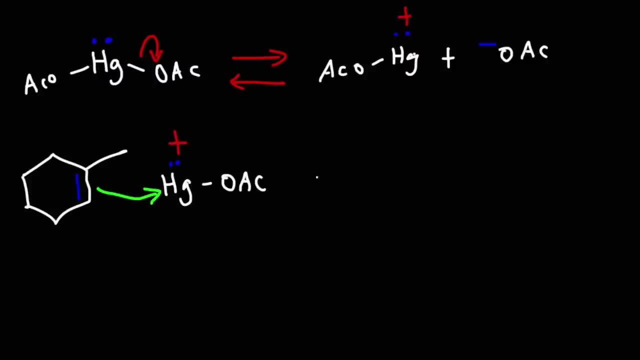 from the nucleophile to the electrophile. Now the mercury atom is going to go on the less substituted carbon of the double bond, That is, it's going to go on the secondary carbon And initially we're going to have a plus charge here. 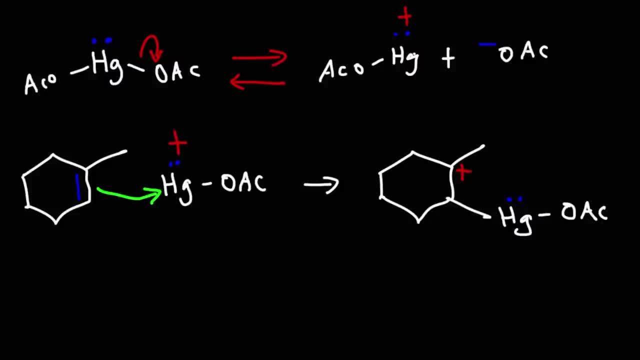 Now you might be thinking this is a carbocation, but it's not, because we do have a resonance form for this structure. This mercury atom can donate a pair of electrons to the carbon with the plus charge, And so we can get a resonance structure. 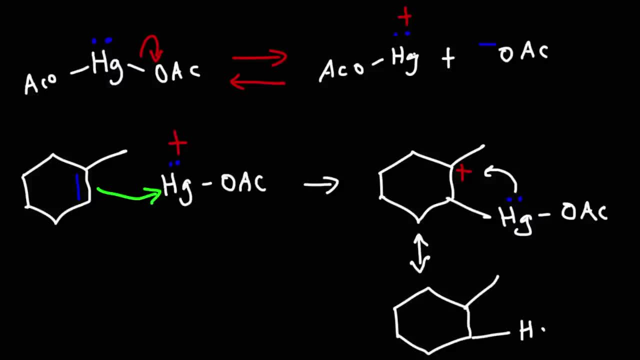 that looks like this: So now mercury bears the positive charge. Now the true intermediate is somewhere in the positive charge, It's somewhere between these two structures. It's not a pure carbocation, because this intermediate doesn't rearrange like a typical carbocation does. 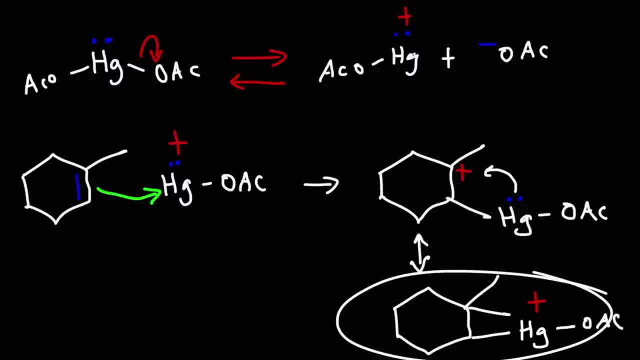 And it's not exactly this structure either, because it does have some characteristics of a carbocation and some characteristics of a three-membered ring, So it's somewhere between the two. So what we're going to do is we're going to draw a resonance hybrid to reflect 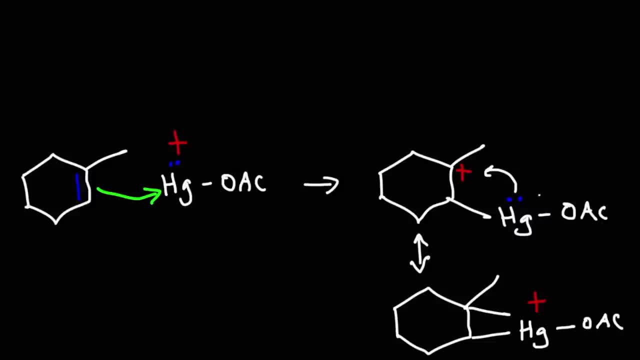 or to get a better, accurate description of the intermediate of this step. So the resonance hybrid is going to look like this. So, since this is the new bond that was formed, we're going to draw a dash for that bond. So we're going to draw a dash for that bond. 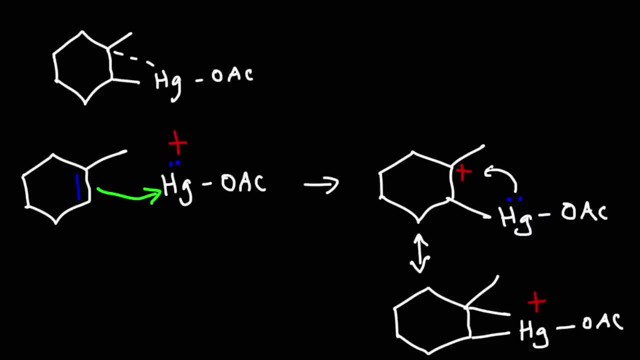 So we're going to draw a dash for that bond. So the plus charge is not completely on this carbon, nor is it completely on the mercury atom, but it's shared between the carbon and the mercury atom. So what we have here is a partial positive charge. 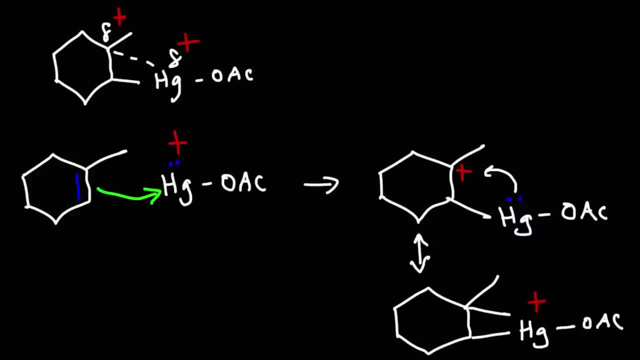 on both the carbon and the mercury atom, So this is known as the mercurinium ion. It's the resonance hybrid of these two. So this particular hybrid explains why we don't get a typical carbocation intermediate for this particular reaction, And it also explains why the nucleophile 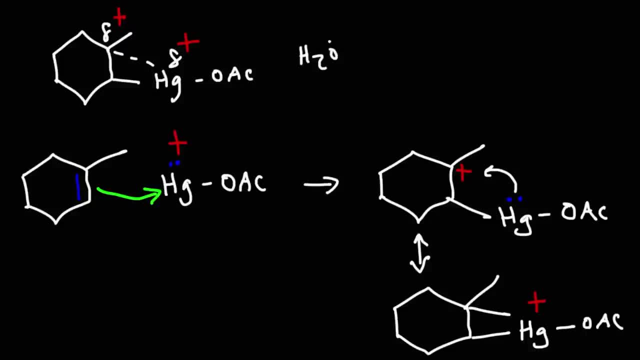 in this case, water reacts with the tertiary carbon as opposed to the secondary carbon. it's because the tertiary carbon has more partial positive charge than the secondary carbon, and so water is going to attack this carbon, and so this reaction proceeds. with Markovnikov retrochemistry. 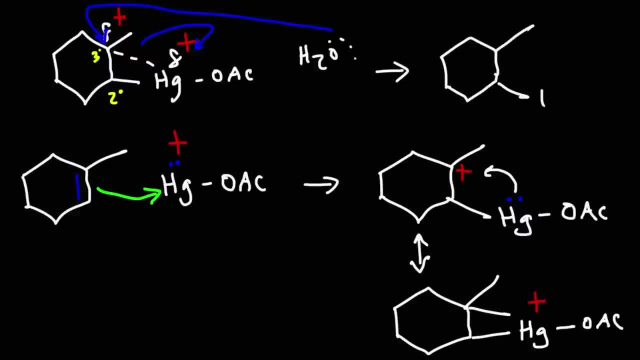 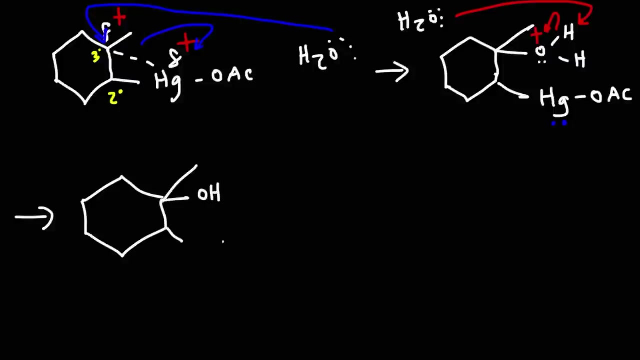 so we'll have our mercury acetate group on one side and on the other carbon. we're going to get an axonium species. now we're going to use another water molecule to take off one of the hydrogen atoms. so going from the beginning to this result, that's the first step. this is 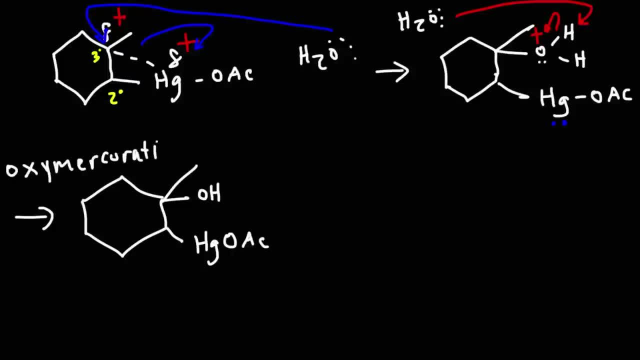 known as oxy mercuration. the second step is known as demercuration. that's when we use sodium borohydride. so the hydride ion will be used to get rid of the mercury acetate group. it's not going to affect the hydroxyl group, so 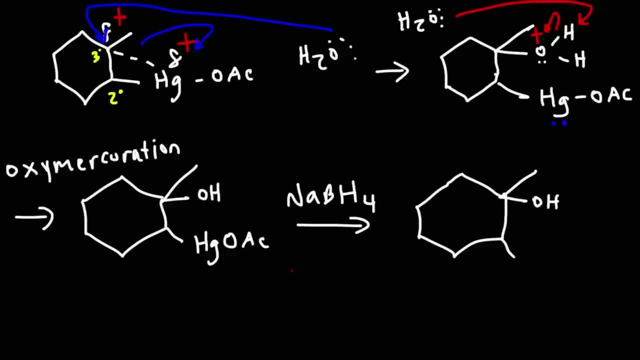 the end result is that we're going to replace this with a hydrogen, so that last step is known as a decarbonization phase, known as a demercuration, that's where we remove mercury and replace it with a hydrogen atom, but the end result is that we get 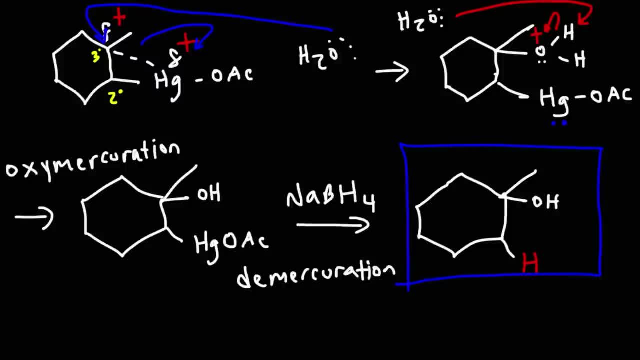 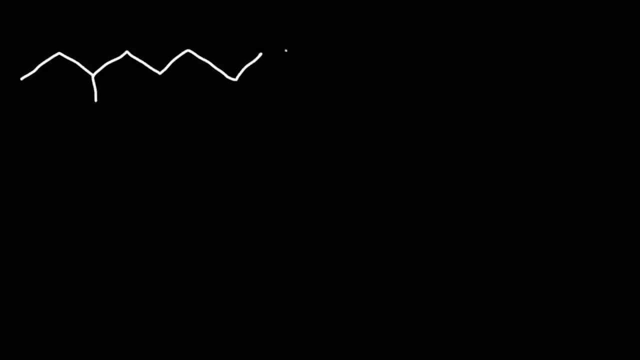 an alcohol in this molecule. now let's work on an example problem. let's say we have two functional groups in one molecule. we have both an alcohol a and an alkene, all wrapped in the same molecule, And we're going to activate this reaction with a dilute amount of sulfuric acid. 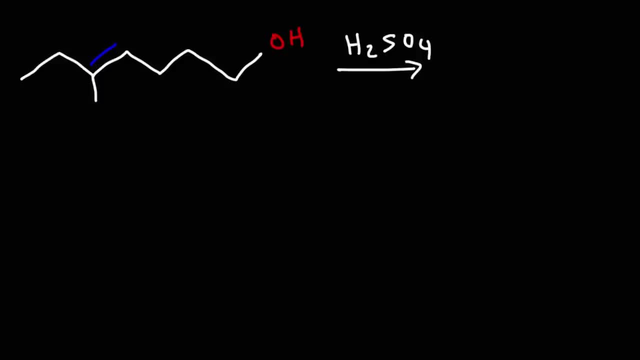 What do you think the product of this reaction will be? Well, the first thing that's going to happen is that the alkene is going to receive a proton from either H2SO4 or from a protonated solvent molecule, And so we're going to get 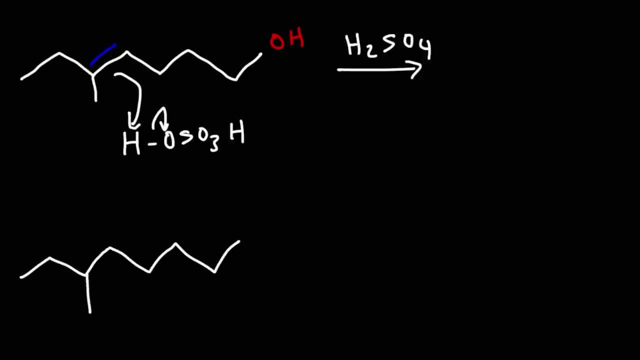 a tertiary carbocation intermediate, Now the hydroxyl group, the OH group, is going to act as a nucleophile. It's going to be attracted to the carbocation since it bears a partial negative charge, And whenever you have this intramolecular reaction, 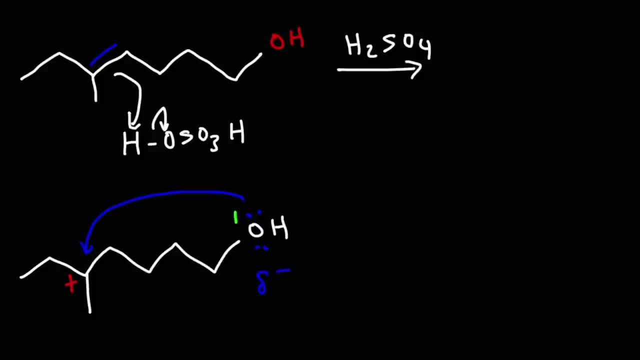 you're going to get a proton And you're going to get a ring. Let's call this number 1, 2, 3, 4, 5, 6.. So we're going to get a 6-membered ring. 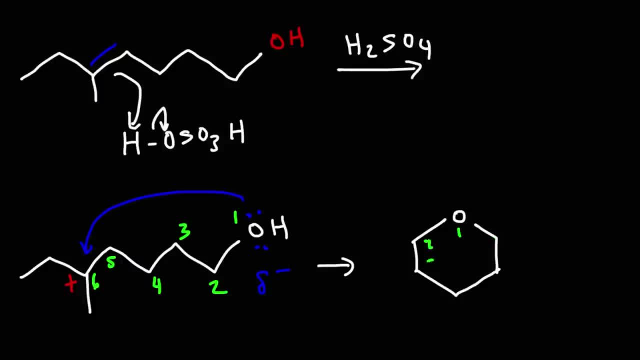 So this is 1,, 2,, 3,, 4,, 5,, 6.. On carbon 6, we have a methyl group And we also have an ethyl group. The oxygen still has a hydrogen attached to it. 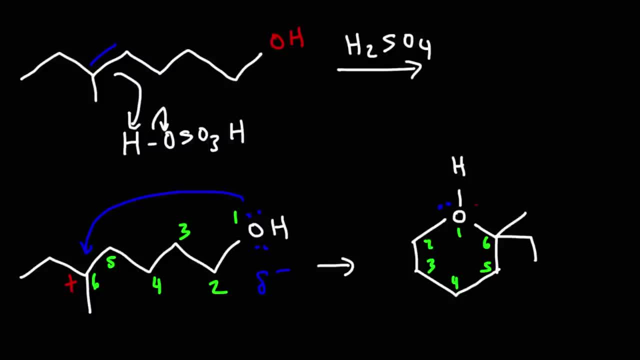 It lost a lone pair, so it has one left over And it has a plus charge. So that's what we have at this point Now: a base. this base could be the OH of another molecule. It could be HSO4- or something else in the solution. 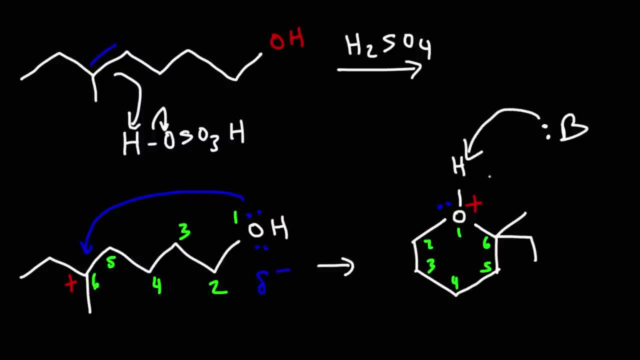 But some molecule is going to act as a base To remove this hydrogen. So the end result of this reaction is a cyclic ether. So whenever you have a molecule with two different functional groups that can react with each other, typically you're going to get an intramolecular reaction. 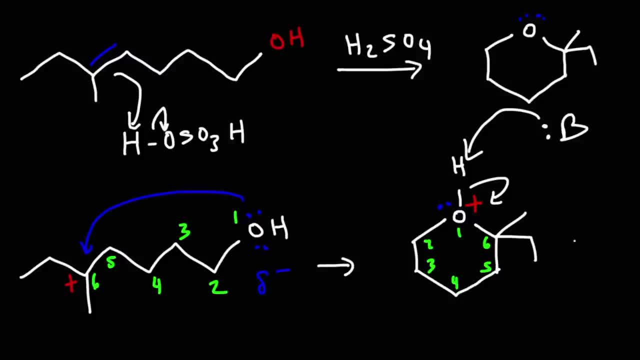 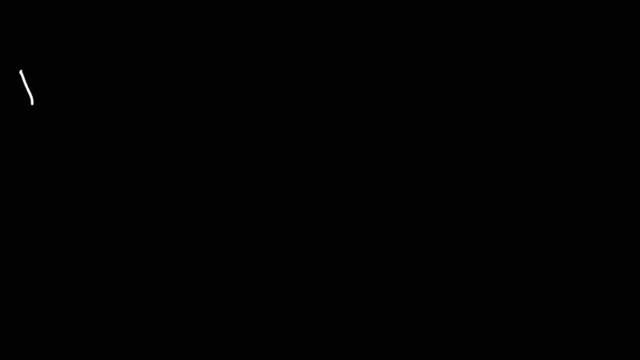 And it usually closes into a ring. So this is the answer for this problem. Now let's work on a few example problems dealing with Hydroboration Oxidation. So go ahead and predict the products for these reactions. So here we have borane and tetrahydrofuran. 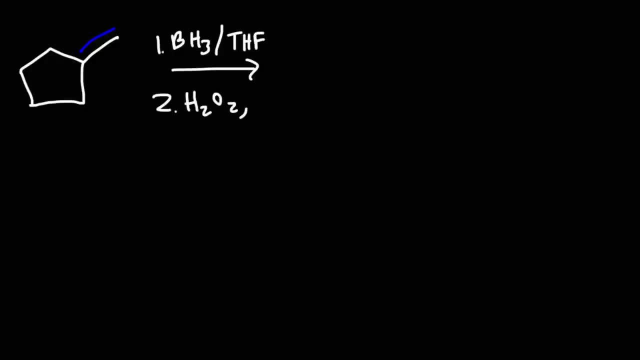 And the second step, followed by hydrogen peroxide and hydroxide. Sometimes you'll see it like that, Other times you'll see water included, But the end result is still the same. And then we're going to compare the product of that reaction to the product of this reaction. 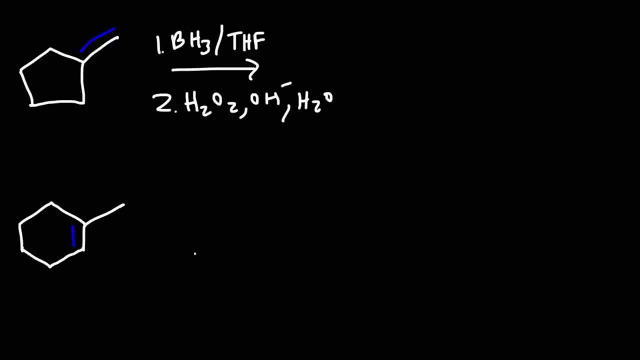 So instead of BH3, we're going to use BD3. Everything else will be the same. So if you don't see water in the second step, the result will still be the same. Go ahead and try these two example problems. So Hydroboration Oxidation proceeds with anti-Markovnikov regiochemistry. 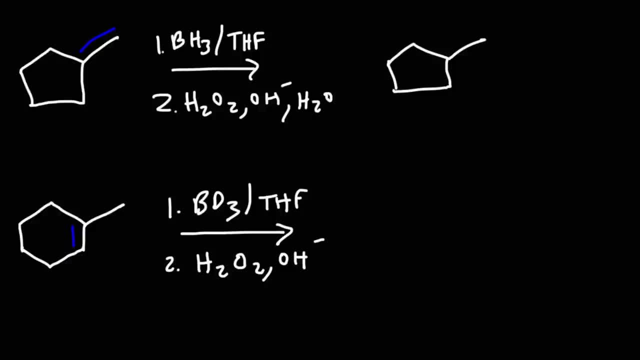 The OH group is going to go on the least substituted carbon atom across the double bond. So in this case that's going to be the primary carbon. So this is going to be the product of the first example. We don't have to worry about stereochemistry. 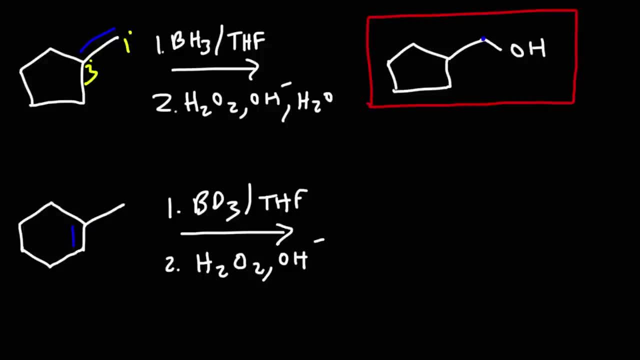 Because, as you can see, this carbon atom is not chiral. Now, what about the second example? For the second example, we need to talk about that. If you see, D, D is deuterium, It's the isotope of hydrogen. 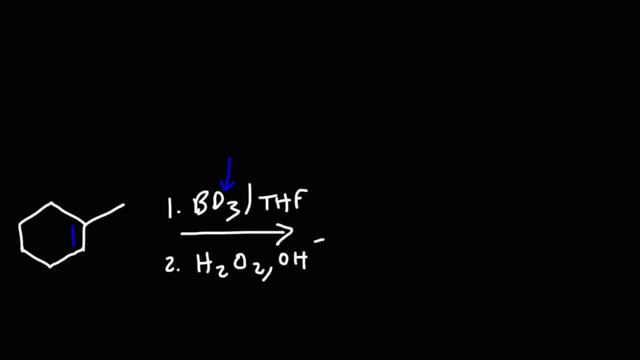 Chemically speaking, they react in a similar way, But they have different nuclear properties, But treat deuterium as if it was hydrogen. The only difference, though, when dealing with deuterium versus hydrogen in organic chemistry, is that in line structures you need to show deuterium. 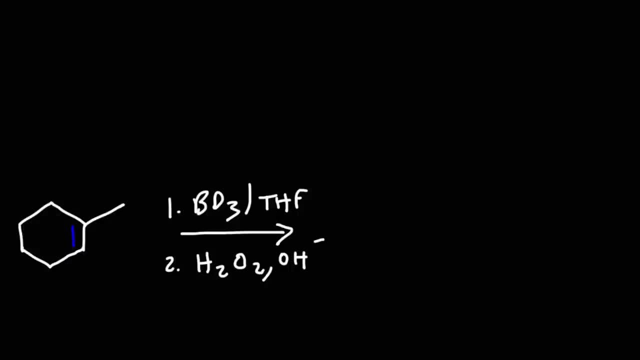 For hydrogen, you don't have to show it, And so that's going to be the key difference there. So let's work on this one step at a time. The first step is hydroboration. That would be BH3 and THF. 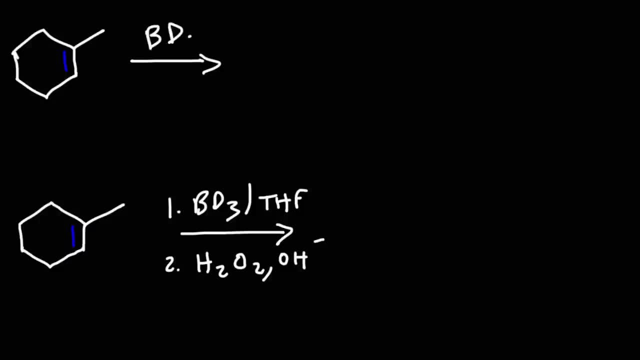 But using BH3, I'm sure it's going to be called something slightly different. Now, during this step, what's going to happen is we're going to add deuterium on the tertiary carbon And BH2 is going to go on the secondary carbon. 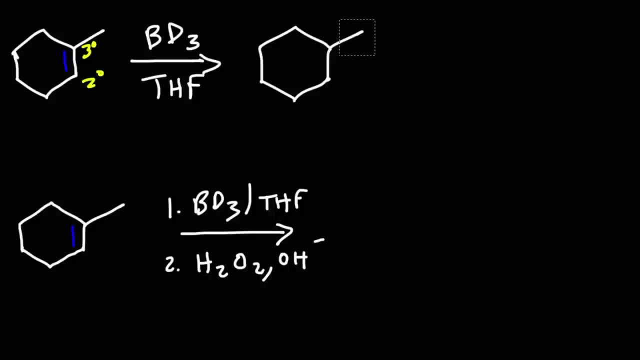 But now we need to highlight this step. So let's say we're going to add deuterium on the tertiary carbon. So let's say the methyl group is in the front, Deuterium will then be in the back And BH2 will also be in the back. 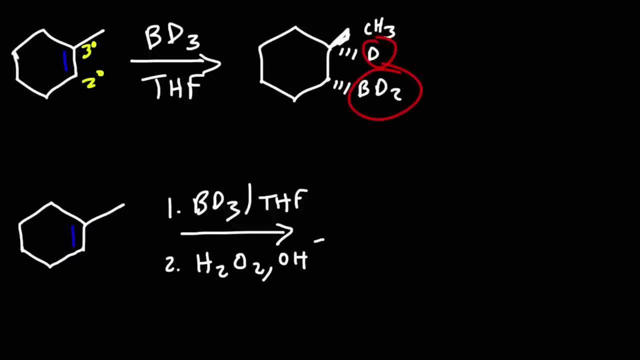 These two groups are added on the same side. This is called syn addition When they're added on the same side. To show the mechanism for that, here's what you can do. So we have deuterium boron and two other deuterium atoms. 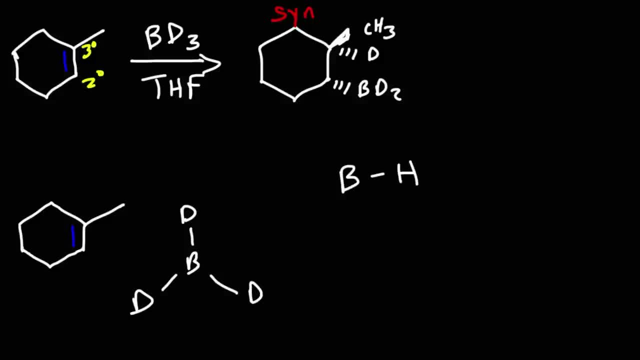 Now, hydrogen has an electronegativity of 2.1.. Boron is 2.0. So hydrogen is slightly more electronegative than boron. So boron is going to be 2.0.. So boron is going to be like the electrophile. 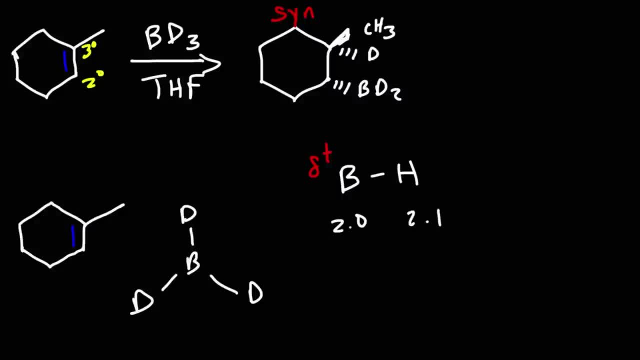 It has a slight partial positive charge relative to hydrogen. Hydrogen is the nucleophile. So because boron is relatively electrophilic, the double bond is going to attack. boron Deuterium is going to be relatively nucleophilic with respect to boron. 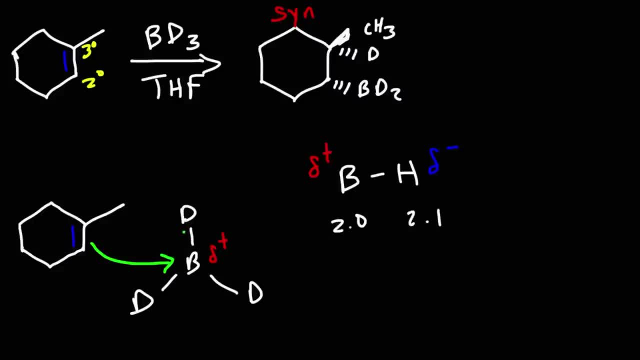 So the bond between boron and deuterium that's going to be used to connect deuterium with the tertiary carbon. So that's how you can show the mechanism. So that's how you can show the mechanism for this first step. 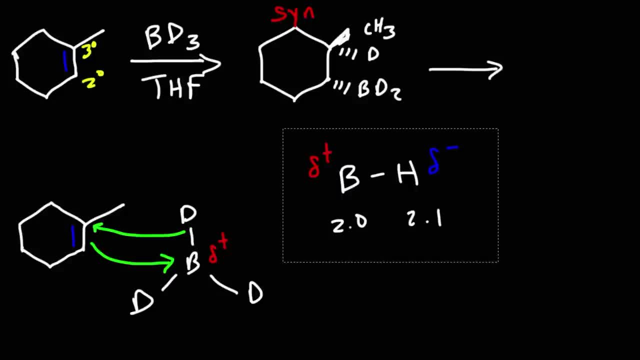 Now in the next step. by the way, during the first step we get this plus the enantiomer. So I'm going to put plus EN for the enantiomer. In the next step, which is oxidation, we're going to oxidize it using hydrogen peroxide. 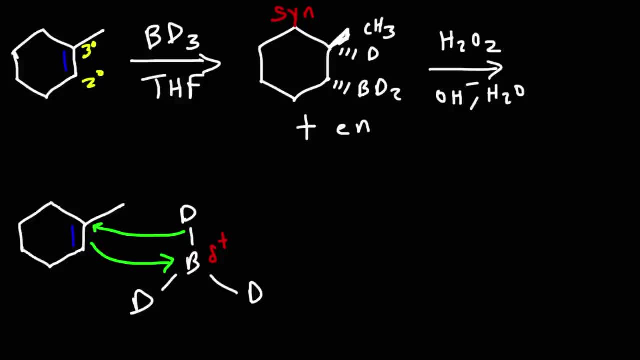 And this is going to occur under basic conditions. So we're going to replace this group with an OH group And it's going to happen on the same side. So if BD2 is in the back, the OH group will be in the back. 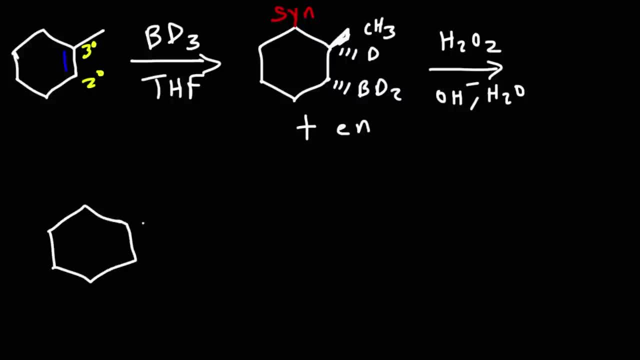 So once we replace it, the end result will be this product. Now we can also get the enantiomer, which is going to look like this. So the end result of the hydroboration oxidation reaction is that the two groups that were added. 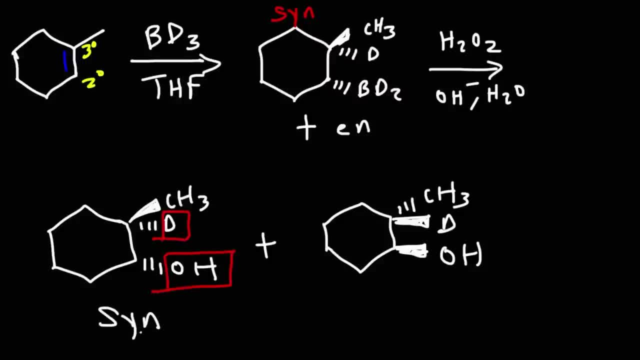 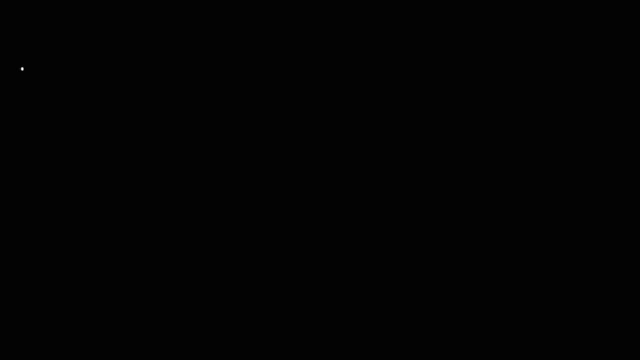 they're added on the same side. So this is a syn addition reaction, And we do get a pair of enantiomers for this particular example. Now let's move on to our next example. So instead of using deuterium, we're going to go back to hydrogen. 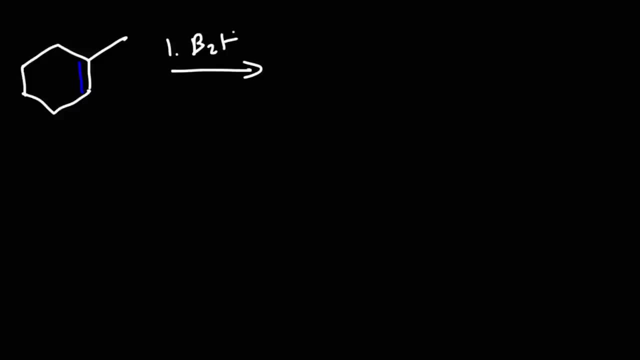 So in the first step, this is going to be B2H6 in THF. By the way, THF tetrahydrofuran is basically a cyclic ether. It's a five-membered ring with four carbons and one oxygen. 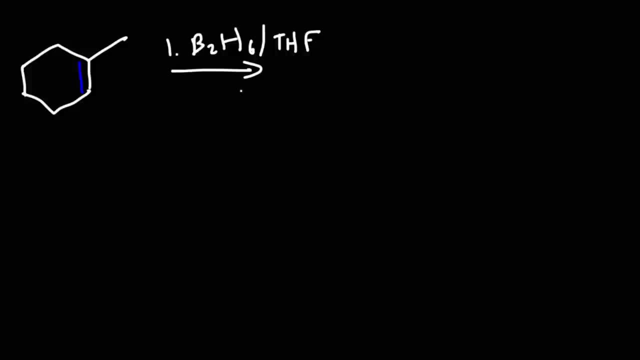 In the second step, we're going to use hydrogen peroxide and hydroxide. So what's going to be the envy zone of this reaction? Now, if you see B2H6, it's going to have the same effect as BH3.. 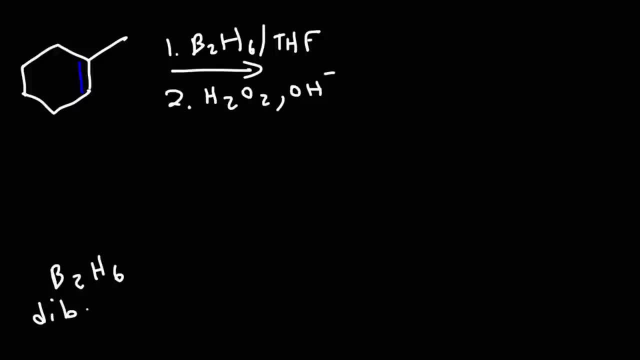 B2H6,. this is diborane. It's basically a dimer of two borane molecules, So this is how it looks like. So here are the two borane molecules, And two of the hydrogens will be shared by the two borane molecules. 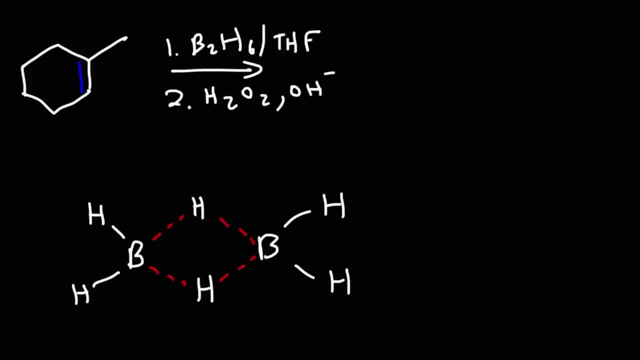 And so that's diborane. It's basically BH3 times two, So it's B2H6.. So what do you think the end product for this reaction will be? We know the hydroxyl group is going to go on the secondary carbon. 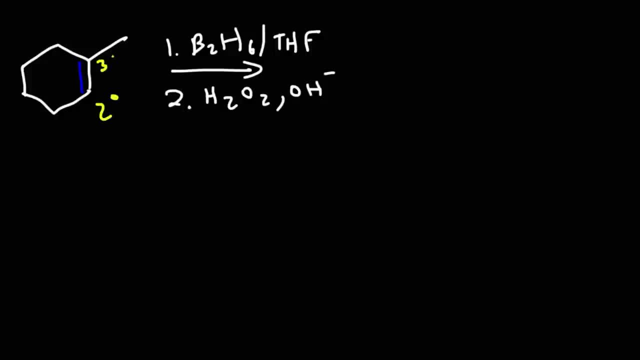 The hydrogen is going to go on the tertiary carbon, So we're going to add hydrogen instead of deuterium this time. The end result for this reaction, with stereochemistry included, is this: So let's say the methyl group, If the methyl group is in the front. 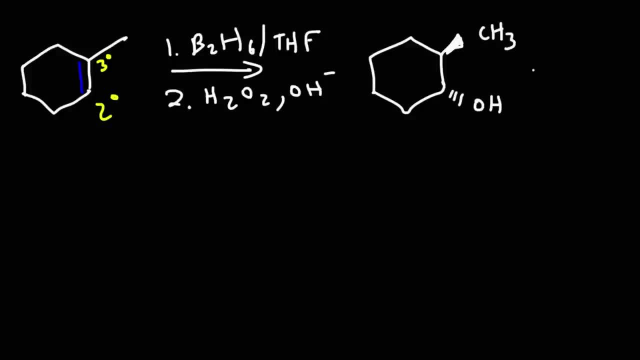 the OH will be on the secondary carbon, but it's going to be in the back And we're going to get the enantiomer as well. So if the methyl group is in the back- and I'm running out of space, so let's put this somewhere else- 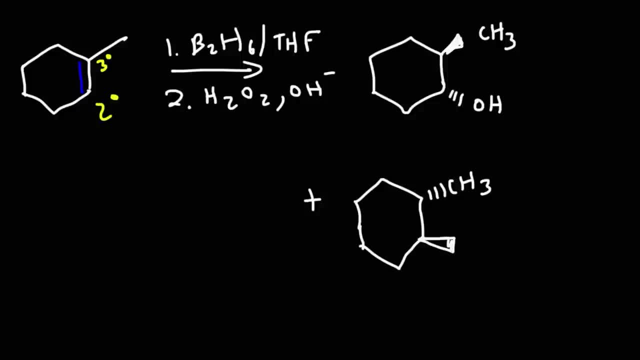 If the methyl group is in the back, the hydroxyl group will be in the front. Now, if you just look at this the way it is, you may think: well, this appears to be anti-addition, Because the methyl and the OH group 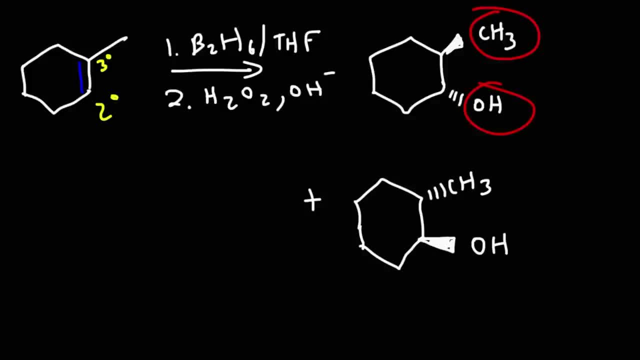 they seem to be on opposite sides rather than on the same side. But remember, we didn't add the methyl group. What we're adding is the hydrogen and the OH. So right now there's no hydrogen here, But the product does have a hydrogen. 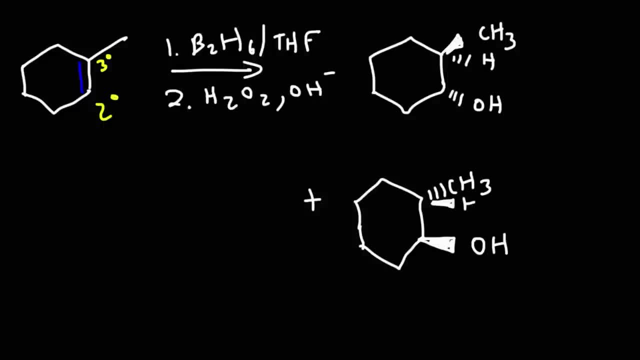 If you show the hydrogen, then you can see that this reaction is syn addition. So these are the groups that we're adding, And those two groups are on the same side, But for a multiple-choice test you won't see the hydrogen. 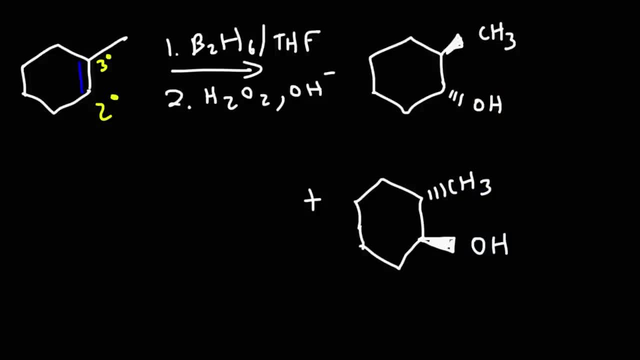 Your answer will look like one of these two, So you need to be aware of that when taking a test on this particular reaction. Now let's go over the mechanism of the hydroboration oxidation reaction. So if we were to react, propene, 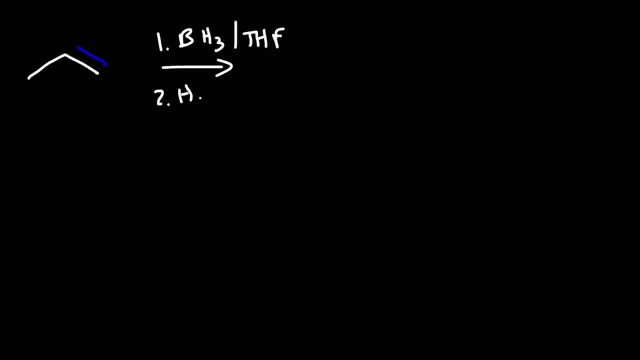 with borane and THF, followed by hydroxide, hydrogen peroxide and water. the end result is that we're going to get an alcohol on a primary carbon, So we're going to get one propanol. But let's show a mechanism. 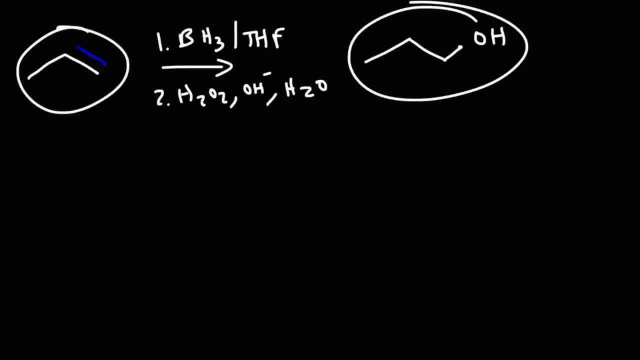 starting from this alkene to this product. Feel free to try it if you want to. So in the first step, we're going to react this with BH3.. And we can draw it this way: The double bond is going to act as a nucleophile. 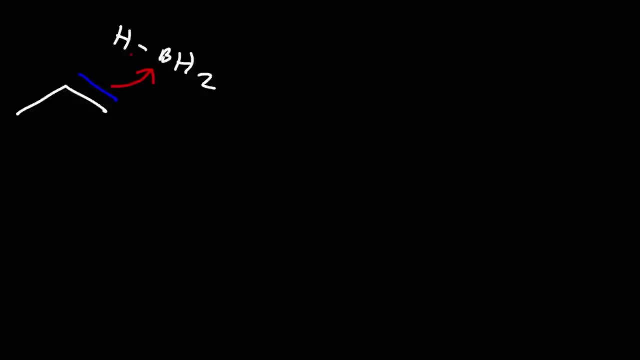 And it's going to attack boron, which is the electrophile, And hydrogen is going to behave as a nucleophile in this case. So we're going to get this product at the first step. We really don't need to show this hydrogen. 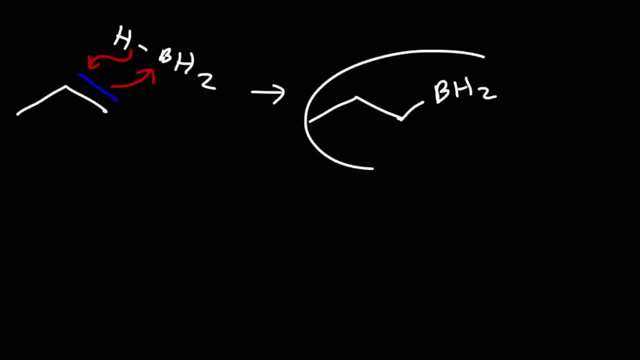 Now this molecule is going to react with another alkene, So I'm going to redraw that molecule here. So we have hydrogen, boron, hydrogen, and then here's the three carbons that we added to the first boron group. So this process is going to repeat itself. 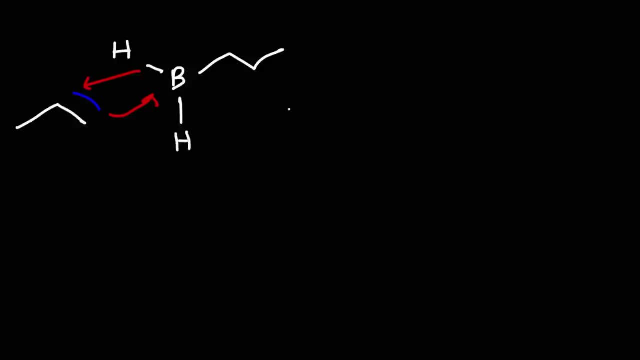 three times. And so now we're going to get another alkene And we're going to react it with the product of this reaction. So the product of that reaction looks like this: now We have two R groups on the boron. 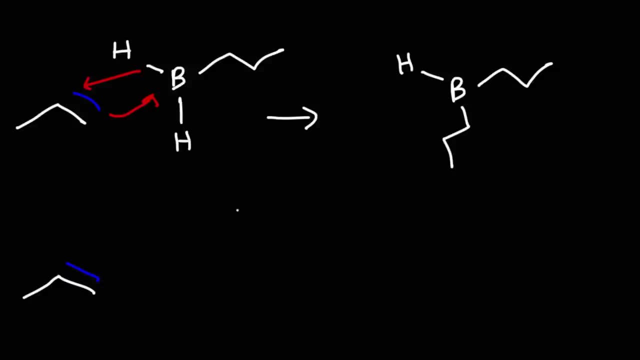 And it has only one hydrogen left over. Maybe it's better if you see it this way. This hydrogen is now here for those of you who might be curious about it. So now let's react to this alkene with this molecule. 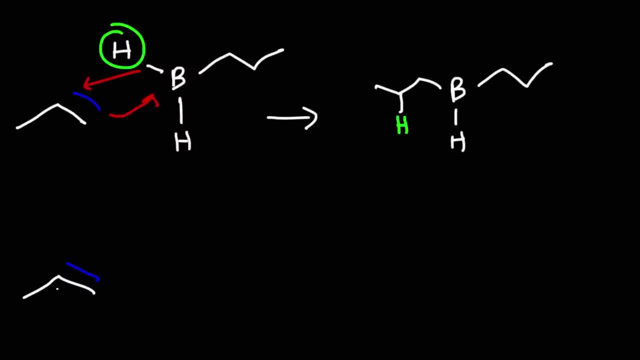 So this hydrogen- I'm going to show it right here- It's attached to boron And boron now has two R groups. So, just like before, the alkene is going to attack the boron atom And the hydrogen is going to connect. 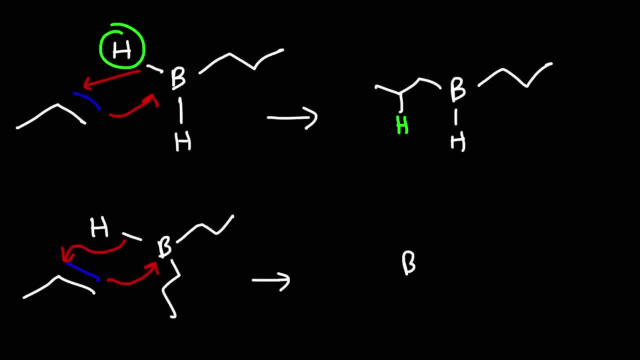 with the other carbon. And so now, at this point, we have a boron with three different R groups. So we have a trialkyl borane molecule. It's trialkyl because there's three R groups. So what we're going to do at this point? 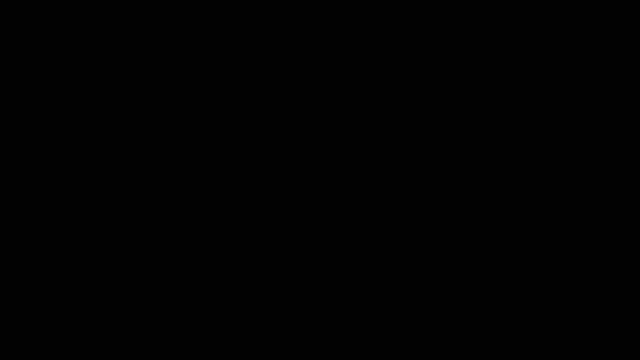 is, we're going to take our trialkyl group. I put too many carbons on that part, So we're going to react to this with hydrogen peroxide. Now, mind you, in the second step, let me just show it here. 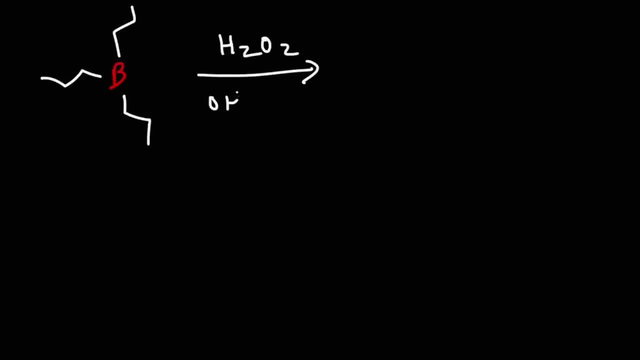 We have H2O2,, hydroxide and water, So these two will initially react. So this is hydrogen peroxide And we're going to react it with hydroxide. Hydroxide is going to remove the hydrogen from hydrogen peroxide. 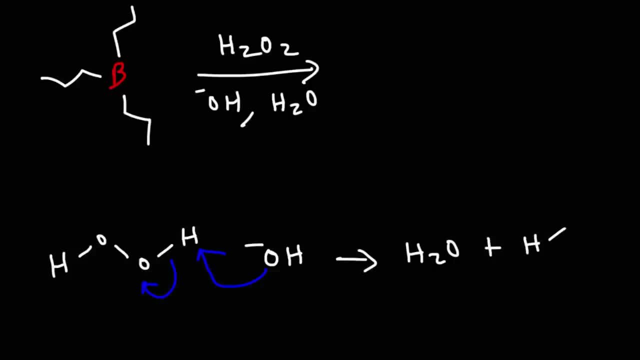 This is going to produce water And this deprotonated peroxide ion. So this part is going to react with the trialkyl borane molecule. 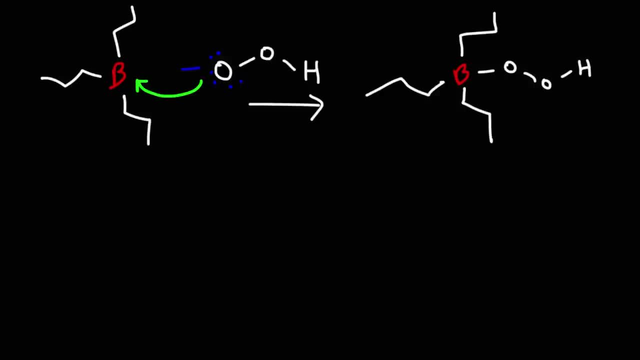